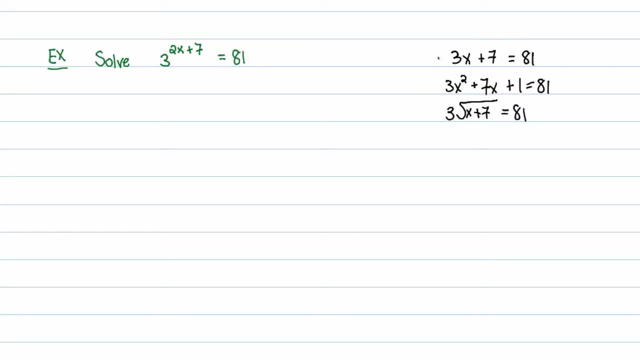 The reason why is? well, ask yourself how you would solve this first one. It has one variable within the entire equation, so you can untie the knot. In other words, you rely upon undoing what's happening to x. So let's see, you would undo a multiplication by three. So in this case you would do 3 times the square root of x plus 7.. 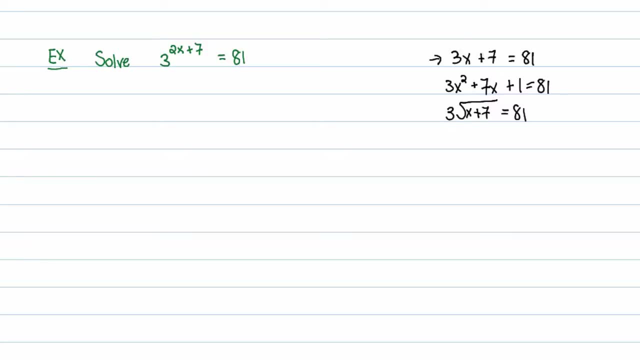 This would be an infinite number, right. So, for example, I'm going to do the same thing here. I'll just give you a step by step, and then we'll do the rest by three. so that involves division. I could do that and you have to undo an. 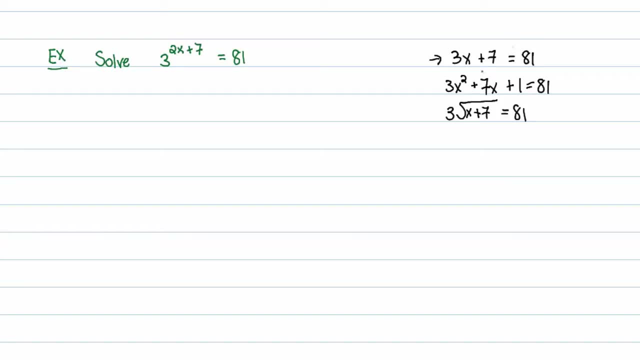 addition by seven. that involves a subtraction. I could do that, so I could easily solve this equation. I'm gonna skip the second one for a moment and go down to the third one down here. the third equation also has only one version of a variable, which means I can untie the knot. you just ask yourself again. 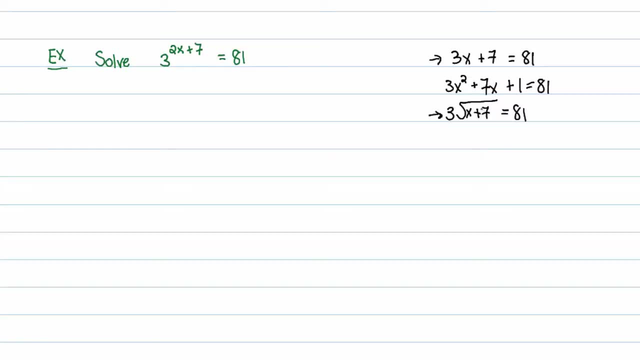 what's happening to X? well, they add seven. so I'll do the inverse of that which is subtract seven. they take the square root of both sides, or at least the square root of X plus seven. I will do the inverse of the square root, which is squaring both sides. they multiply that by three. I'll do the inverse of. 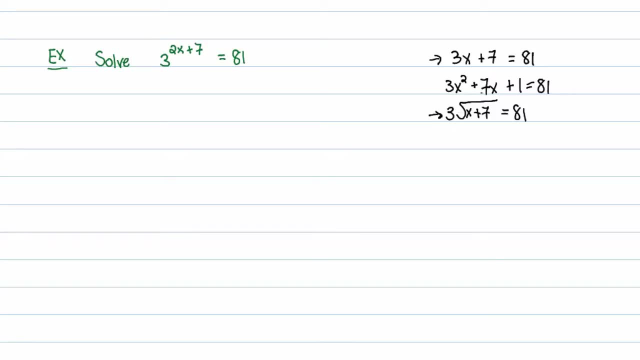 multiplication by three, which is division by three, this middle case here. this is a special scenario. so you have 3x squared plus 7x, and then plus some number equals some number. these two terms cannot combine, so you have to resort to special techniques. the special techniques. 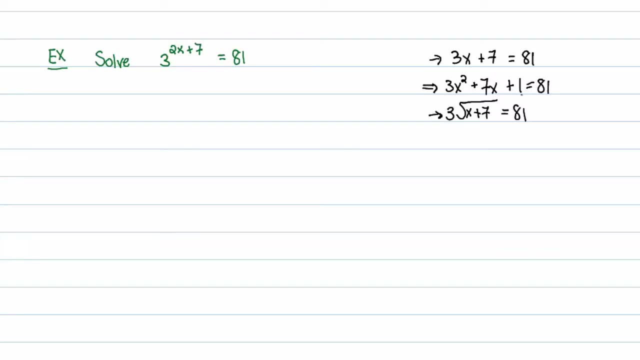 here are the ones that I'm going to talk about in a minute, and then I'm going to go back to my own course. I'll explain them in a minute, but I'd rather than this- I'll just go ahead and get started. so what I've done on the first number. 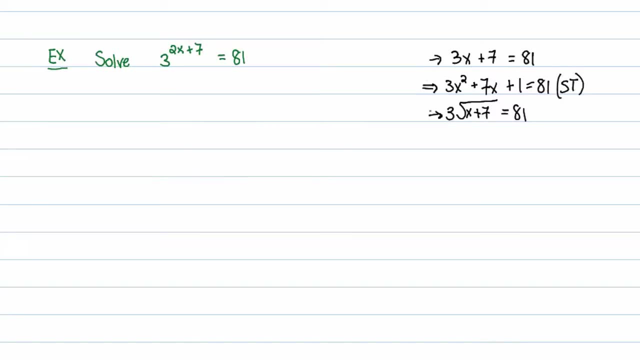 is. I've done this math line. so first you lashes out your algebra becomes a vector that the squared square root of the square root of t. so what I'm going to do is I'm going to go to my math problem and go over to my own course, to 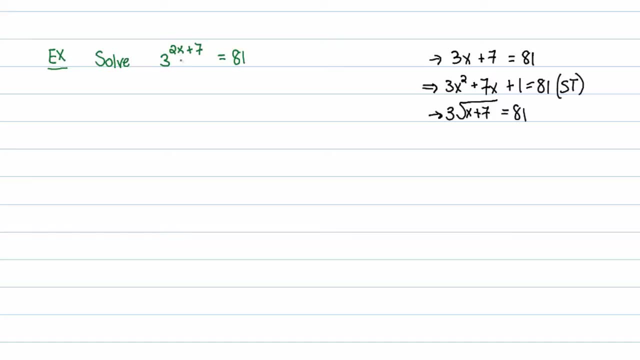 be able to find my elections, and then I'm going to go to my formula, and then what I'm going to do is I'm going to go over and I'm going to go back to my do. what i normally do is, which is ask you what happened to x? we start with focusing on x itself. 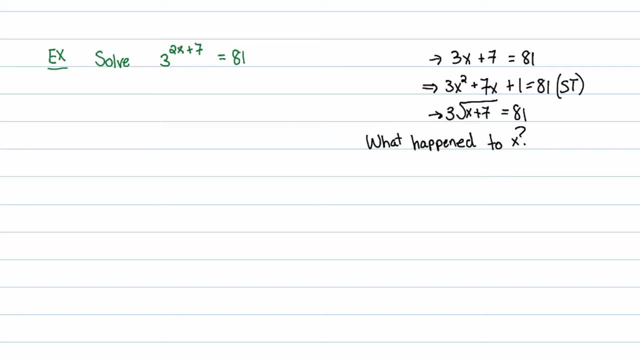 so zoom in, just kind of look at x and say what, what's the first thing that happened to it? well, first thing that happened to it is it got multiplied by two. and the second thing that happened to it after it got multiplied by two is somebody added seven to it. both of those i can undo. 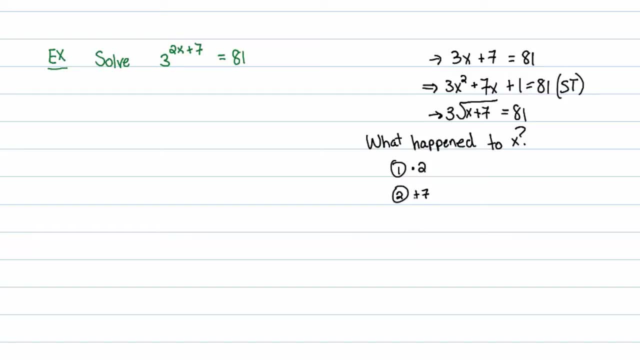 i can divide by two and subtract seven. i can do and do those. but the third thing that happened to this picture- two x plus seven- is it got raised. it is the exponent with base three, so it got raised. it is now in this type of structure and i have no idea how to undo that you can't normally. 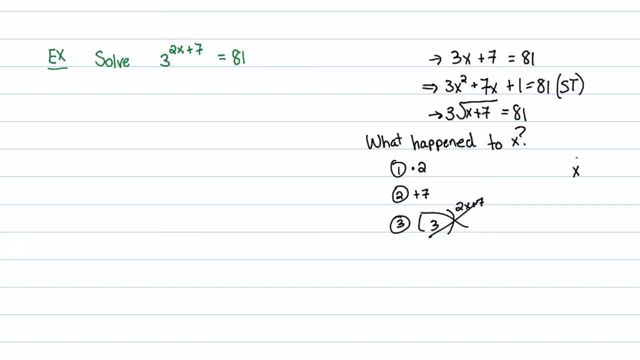 uh, so i'm going to cross that out. normally, if it was like x to the third, i can undo that by taking the cubed root. see those powers undo each other. but you have three to the two x plus seven and i would be totally confused if i took the two x plus seventh. 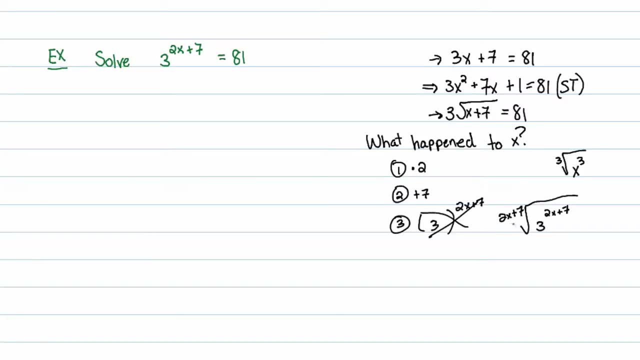 root, even though they would cancel. i still don't know what the two x plus seventh root is, so very bad idea. so right now i have no idea how to undo or basically unlock an exponent. i can't unlock a variable from an exponent yet, so my only choice is to hopefully. 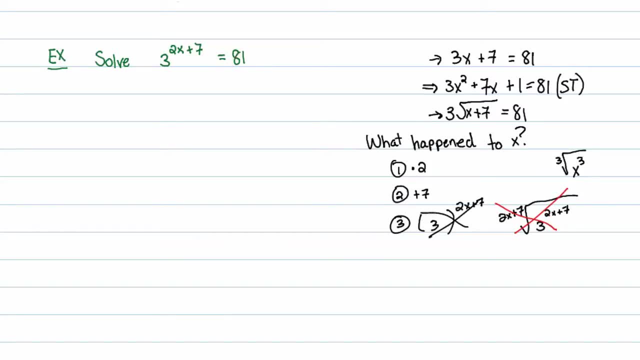 get this eighty one as a similar number or as a exactly the same number, but just a different representation. what i'm looking for is to use the following theorem: if you have a base b, that's supposed to be a b, i kind of butchered it- b to the mth power and it equals that same base to the. 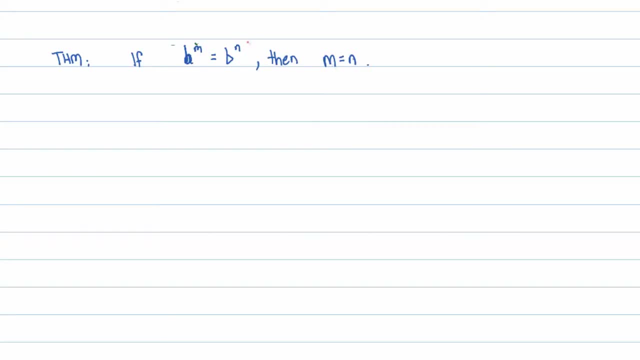 nth power, then you know, those two powers have to be the same: m has to equal n. so i'd like to rewrite this equation to where both sides are just exponential expressions with base three. well, this eighty one can be rewritten as three to the fourth power. so let me go ahead and do that. 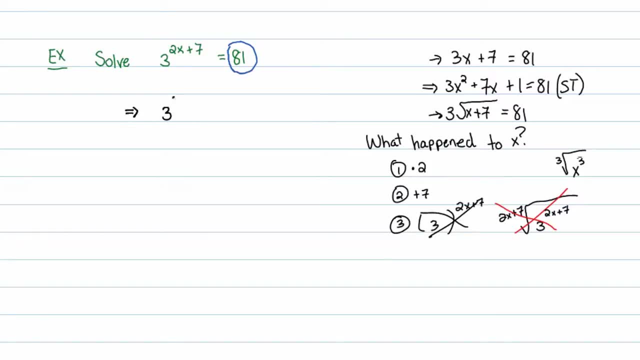 this implies the left hand side- i'm going to leave- is three raised to the two x plus seven power. the right hand side, that's three raised to the fourth power. and now using, since they have the same base, using this theorem, where the base is the same, then they're going to be equal to the third power and 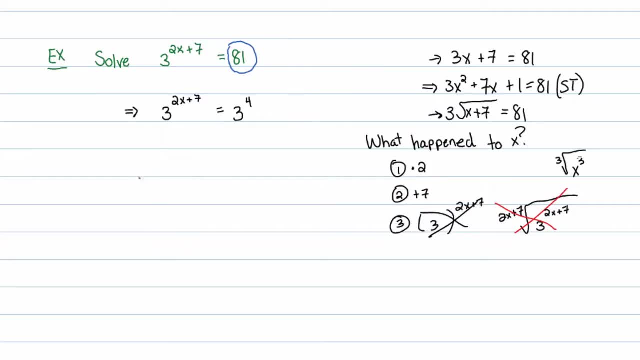 their exponents must be equal. so i'll go ahead and set the exponents equal here. let's see: two x plus seven must therefore equal four. and now this i can easily solve right: subtract seven, divide by two and we get this: x is a negative three halves. 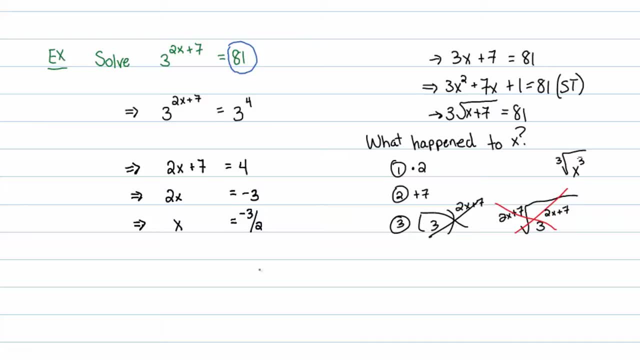 that's how you do it. this is how you solve all these exponential style problems where you, if you don't know what a logarithm is. that's how it's done. now, obviously, there's going to be a point- i'll write this in red because this is not for our discussion right now- but there's going to be a point where you have like: 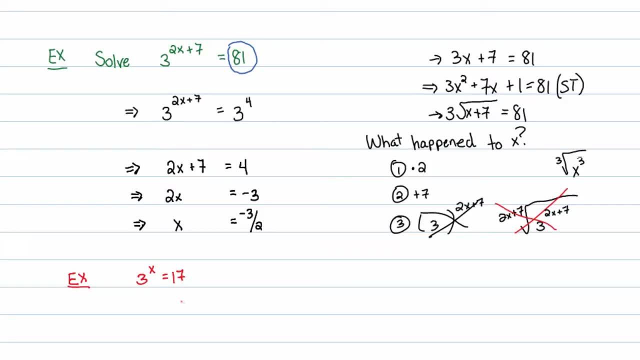 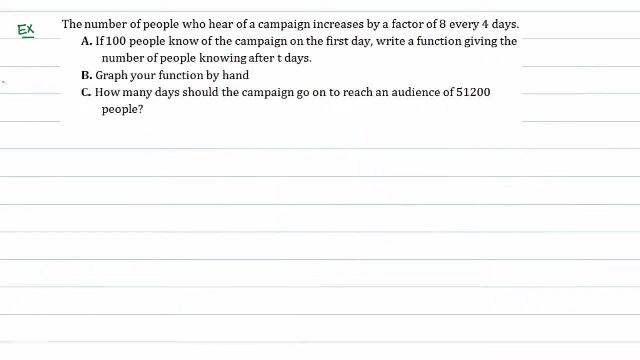 something like three to the x is equal to seventeen, and you cannot write seventeen easily as three to a power. it's not very easy to do so. this you can't do using this method. this requires something called a logarithm. so i'm just gonna- i'm just going to skip out on that right now, because i'll dedicate an entire series of lectures to logarithms. 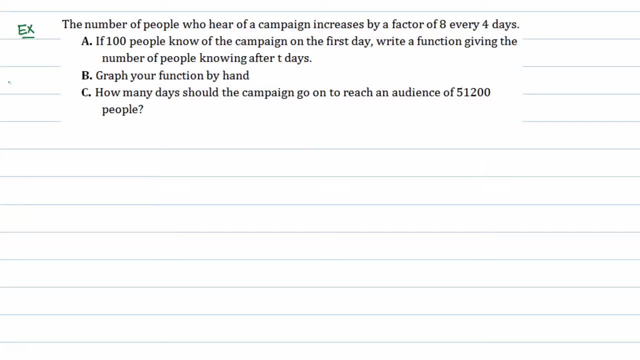 now, even though we don't have the technology of a logarithm, we still can solve a lot of applications that involve exponential functions. let's take a look at this one. the number of people who hear of a campaign increases by a factor of 8 every four days. 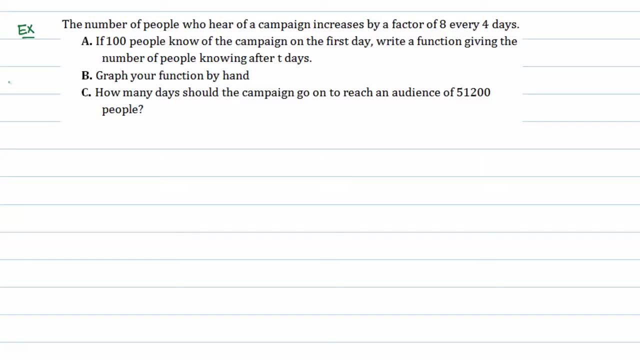 so that's the important part here. here is that they- that's kind of their way of telling us- a growth factor. so that's why you need to know everything about exponential functions prior to this lecture. if a hundred people know of the campaign on the first day, write a. 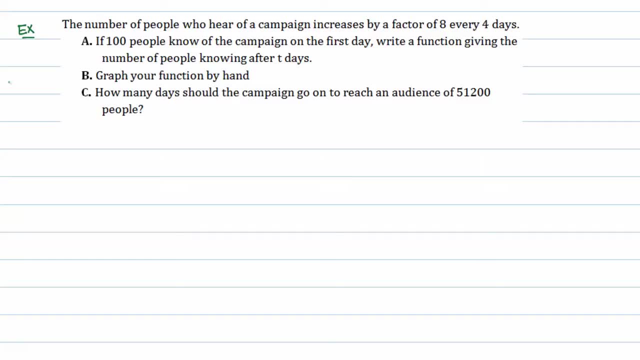 function giving the number of people knowing about the campaign after T days. so let's start there. one thing we do know is that this 100 people that initially know that will be our P naught, and in fact, maybe I should write down the standard form or the, the form of the exponential function I'm going to use. 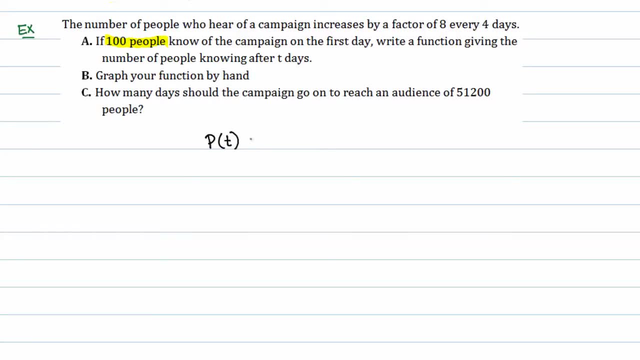 I'll use. P of T is equal to P naught, B to the T. that's the exponential function format there, and P naught is just our initial value, our initial number of people. in reality, this is going to be actually- I'll write it up over here. this will be: 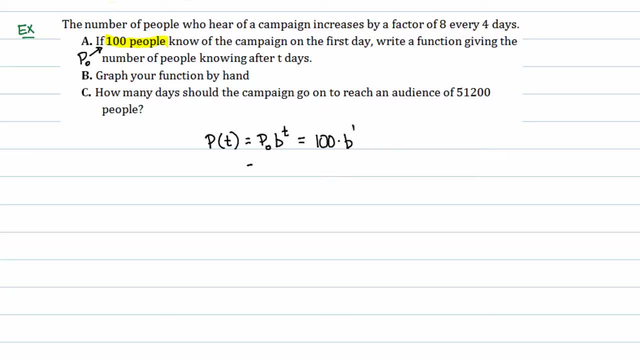 100 times B to the T power. and now all I need to know is what. what is B? well, they tell me that it increases by a factor of 8. in other words, it gets multiplied by a factor of 8 every four days from our work, previous work, with all the function. 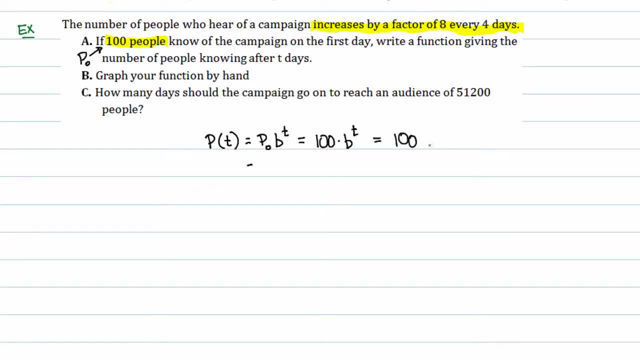 notations and building exponential functions board problems. we know that means that we have something like eight. in here is every single group of days. it gets multiplied by a in the happens every four days, so increased by a factor of a every four days. that's our function, and now I. that was actually part a, so let me just rewrite. 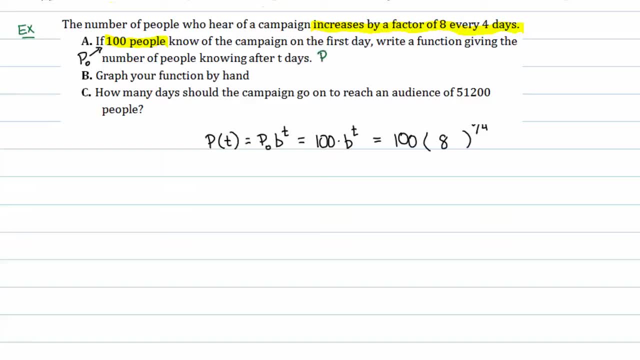 that next to part a, there that we have p of t. so just in case i need to erase this, i don't think i will have to- equals 100 times 8 to the t over 4 power. now graph your function by hand. that's going to. 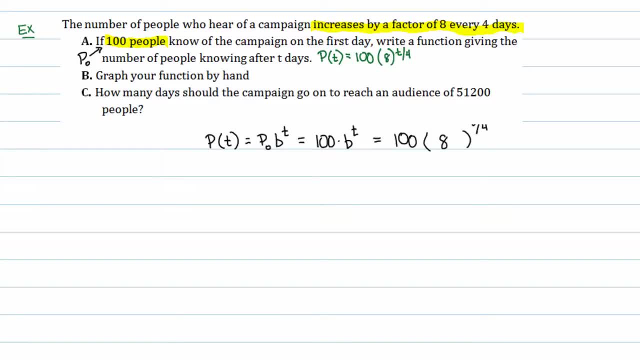 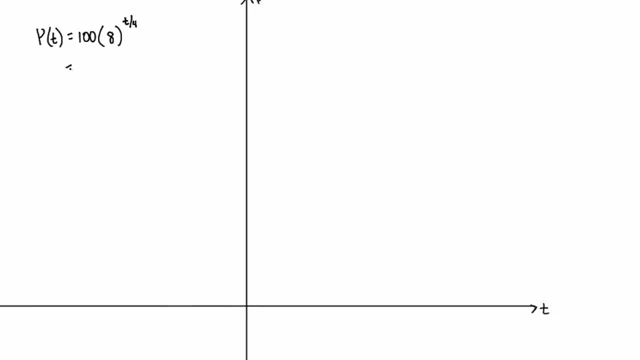 be very difficult to do, but we'll give it a whirl here. so i draw some axes in here and i'm going to go ahead and rewrite this in a graphing format, in other words, a form that's easier for me to graph with. that's like 100 times 8 to the 1, 4th, all being raised to the t. remember: powers to powers. 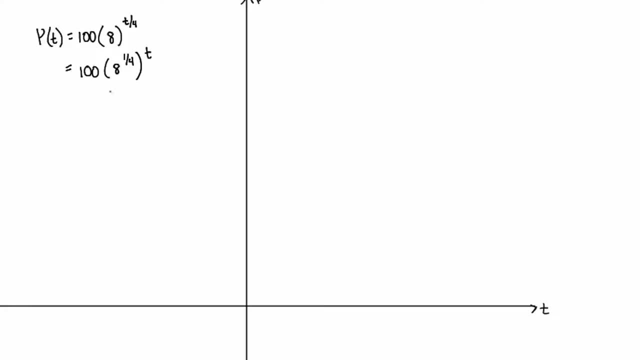 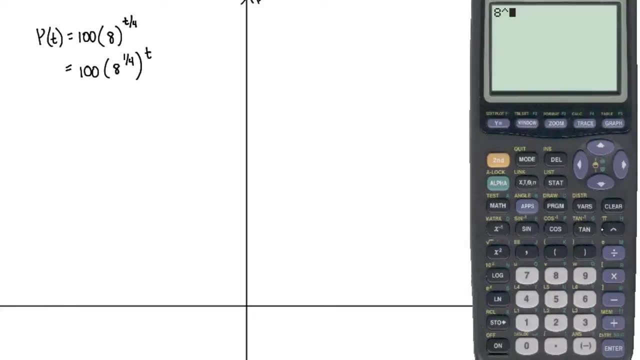 multiply, and then i can use a calculator to figure out what 8 to the 1 4th is, because that's not going to be a nice number. i'll tell you that. so, 8 raised to the 1 4th power, i'll get 1.7. 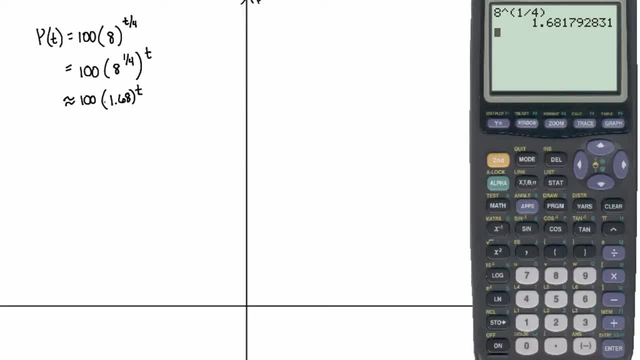 6, 8 roughly, and the reason why i like this format is just because this is how applications are generally handed to you. anyways, they give you some nastiness. there's a lot of things you can take away from this. first of all, this is our initial value. that means, at time, zero. 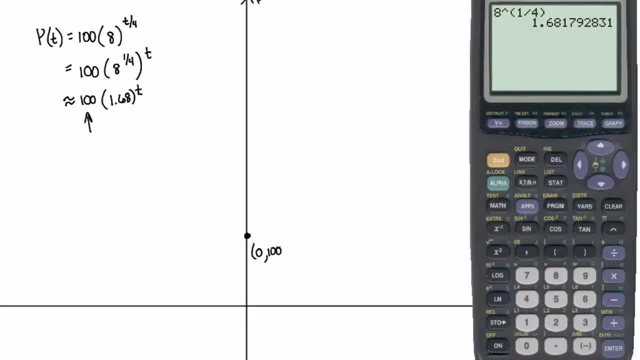 we are at a height of 100 on the vertical axis, so at time zero with 100 people know of the campaign. and then, from that point forward, the it's being multiplied by the number of times divided by powers of 1.68. so it's growing. i'll go ahead and just show how it. 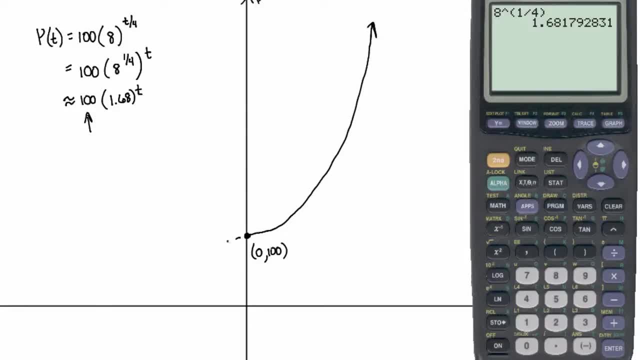 might grow. it might grow something like this, who knows? by the way, technically, if it's an exponential function, it should go this way, but the fact is this is a real application. so we generally start graphing today and we don't concern ourselves with the past. now a really. 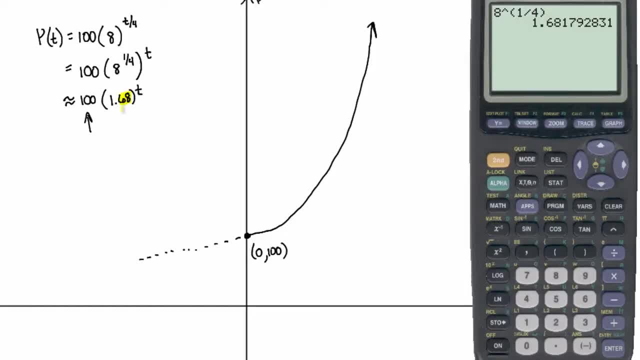 cool interpretation of this number is that this means every day that goes by, the number of people who are people that know increases by 68%, and I'm a big fan of that interpretation. so that's that's just a great thing to know that that when you have something like 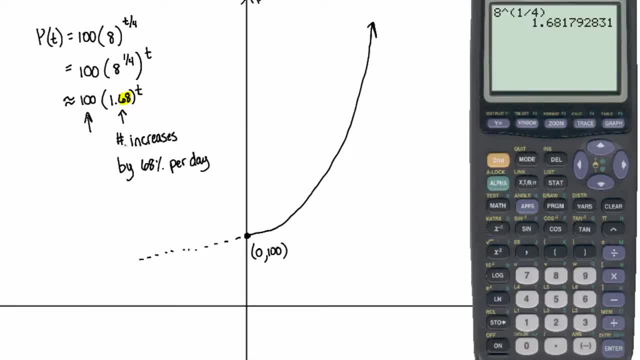 one point number number, then you know that that's a. that's the percentage increase that's happening. now I would like to graph another point so you could choose a value for T. now, like I said, I wanted to kind of write this form out here just so we can get an idea of what the graph looks like. but in reality I'm 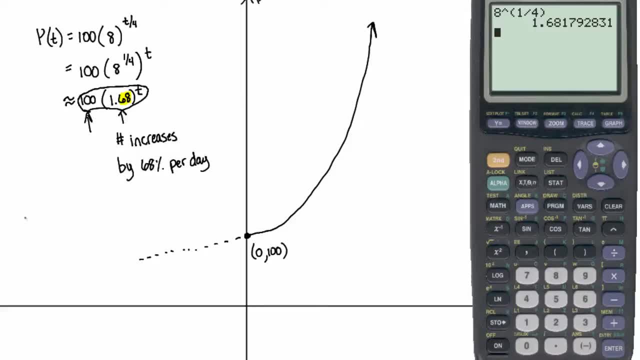 probably just going to choose T equals 4. if I choose T equals 4 in the original function, without all my manipulation with a calculator, I get this 100 times 8 to the 4 over 4 power, or in other words, just 100 times 8, which is 800. so 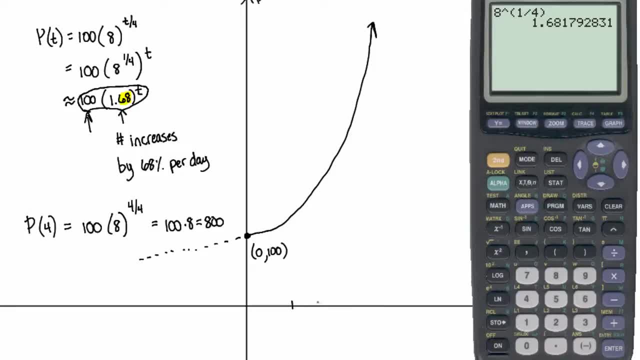 that means at time 4, so maybe 1. well, let's say this is 1, 2, 3, 4, so day 4: 800 people now. now, of course, my graph is not to scale. this should actually be up a little bit higher, but I'm okay with that. 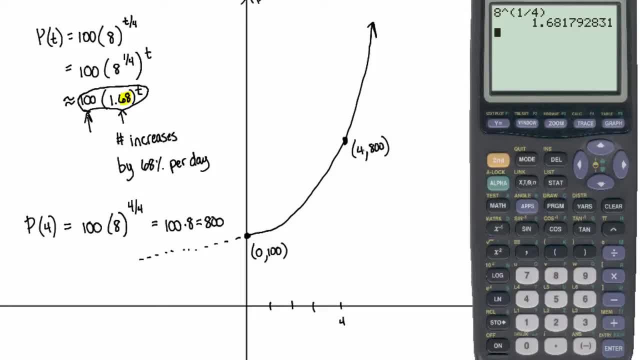 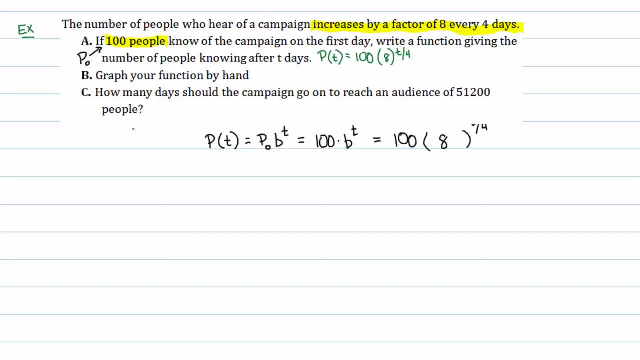 4 comma, 800. good exponential growth on that. now the part C of this problem is a really interesting part. it says how many days should the campaign go on to reach an audience of five, fifty, one thousand two hundred people? remember our function is this: the number of people who know is equal to 100 times. 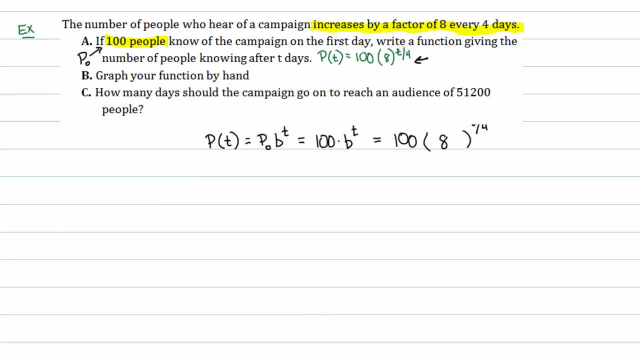 8 raised to the T over 4, where T is the number of days have gone on. we want to know when that number of people is going to be fifty one thousand two hundred. in other words, we're going to let P equal fifty one thousand two hundred. so let's. 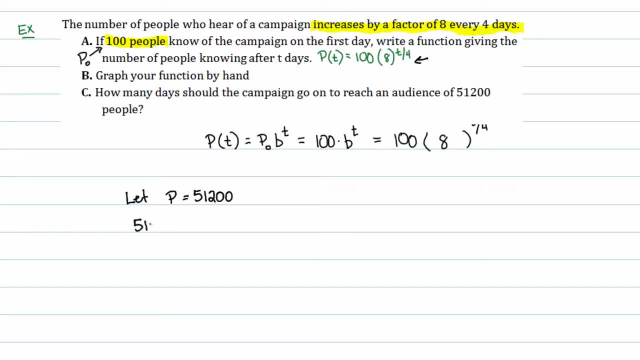 go ahead and do that. fifty one thousand two hundred must equal 100 times 8 raised to the T over 4, and you might think I can't do this because there's just no way I could, I can't, I don't know how to do this. well, 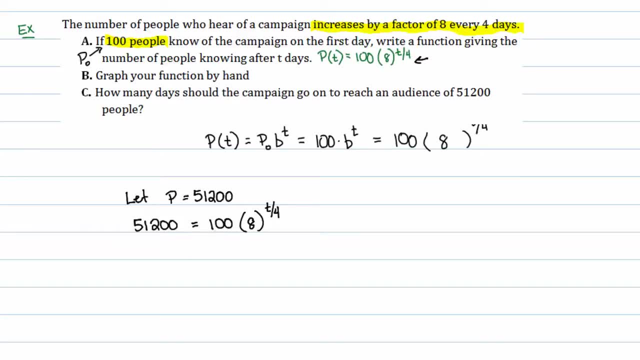 divide both sides by 100. first start easy, start with just these simple, if simple simplifications. I can't talk today, or any day really. 100 over 100 is 1 and of course, 551, 200 is over 100 is just 512, so we go ahead and write that in if 512 is equal. 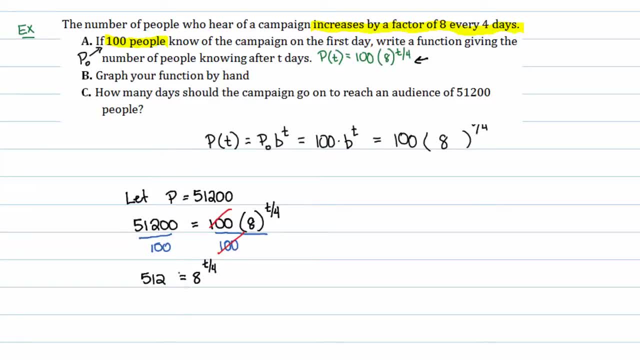 to 8, raised to the T over 4. now, geez, I really love it if 512 was a power of 8, that'd be awesome. if it's not, then I have to resort to powers of well, something that I can write 8 in terms of, if you grab a calculator and you start. 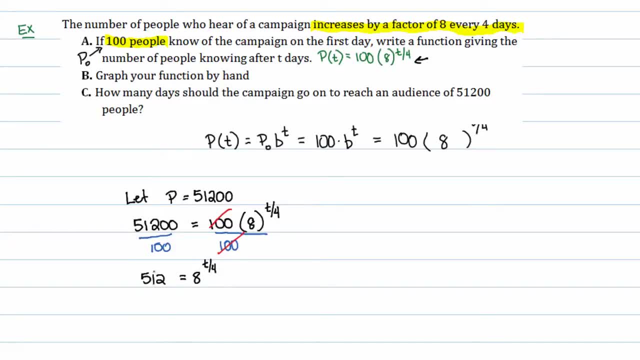 looking for powers of 8, you'll find out that eights to the third power is going to be 512, so this is actually equal to 8 to the third power. now, in a way, this problem is set up a little bit easier than I would like, because 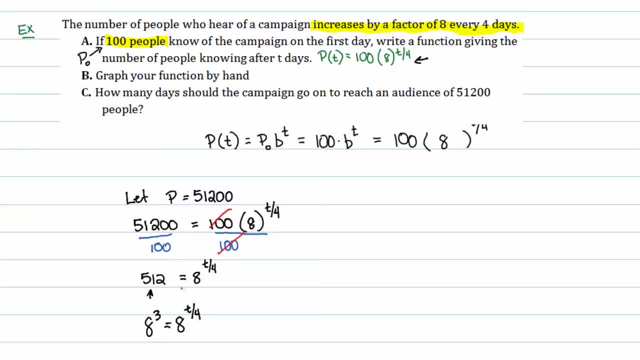 honestly, it'd be nicer if these two weren't so beautiful. it'd be nicer if that. if we had to basically do a prime factorization on both, you can still do that. I could have said: listen, 8 is the same thing as 2 cubed. I could have done that. and on the left hand side, 512 is the same thing. 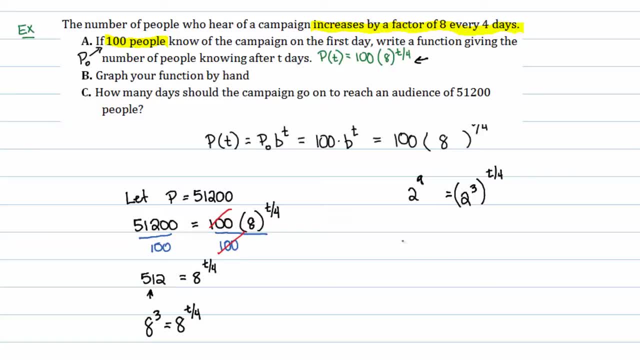 as 2 to the 9th, and now I would rewrite that as: 2 to the 9th is equal, to remember, powers to powers, multiply, so that's going to be 2 to the 3, fourths power, 3 T over 4 power. sorry so, therefore the powers, since the bases are equal, the 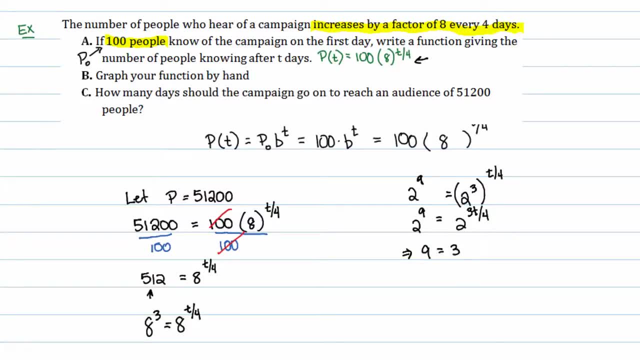 powers must be equal down, then, and the�pげ như மbung that by two to make that problem obvious. instead, we're doing significantYAN sort of alone length and heartbeat here. So in either case, you would have gotten the right answer. 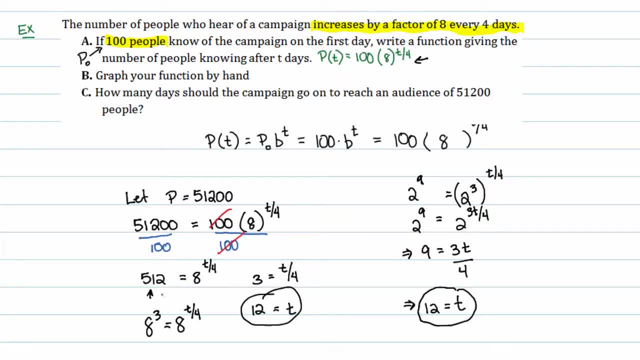 The idea is to wiggle them down to where their primal base. their prime bases are the same like we have here, So we had their prime base on this was just a 2, and the prime base on this was actually just a 2 as well. 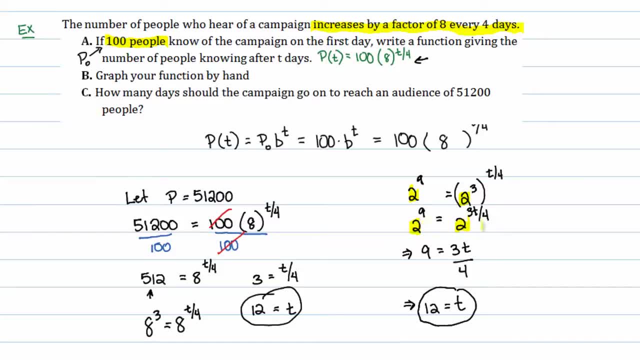 Once you get them written as 2 to a power is equal to 2 to a different power, you can now say those powers must be equal. So this tells me that in 12 days, 51,000. some odd people will know. 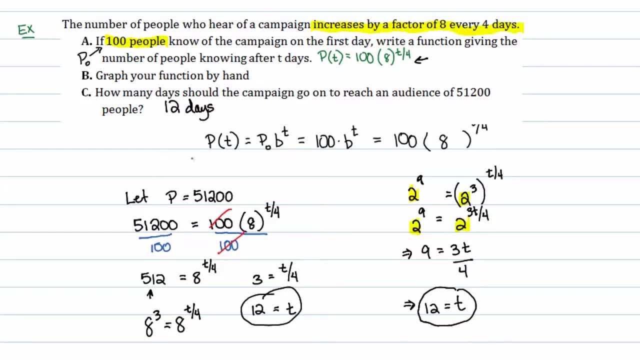 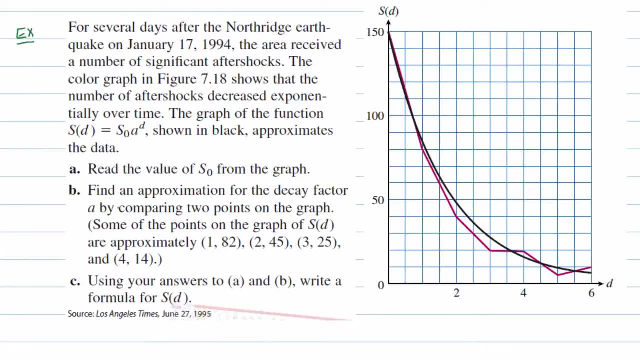 Let's write that in there. That's a pretty short period of time. That's how powers work, though Very neat. Now there's another application for solving equations- exponential equations, This one. I'm going to show you how to use your graphing calculator on. 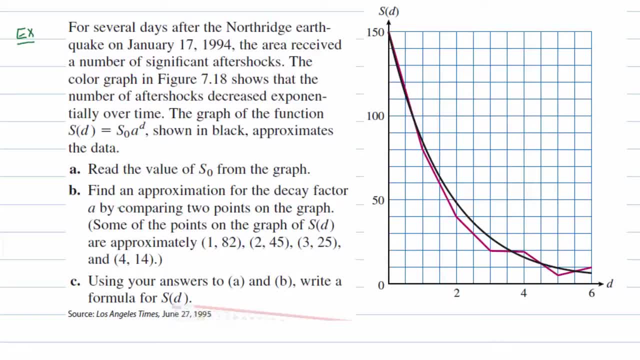 For several days after the Northridge earthquake on January 17, 1994, the area received a number of significant aftershocks. The color graph on this graph over here- the red part of it, I should say- shows that the number of aftershocks decreased exponentially over time. 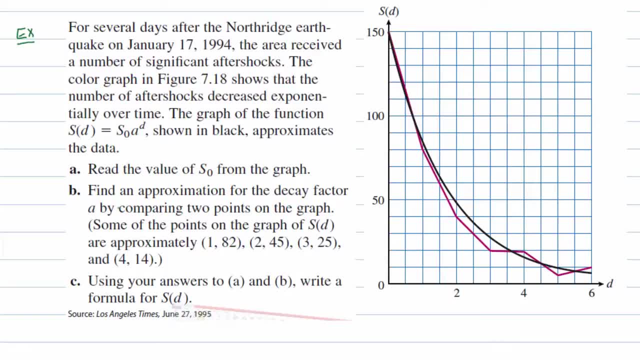 And this data is from the LA Times June 27, 1995.. So it does look like it decreases or decays exponentially, And the reason why is because there's this black curve. that's an actual exponential decay. So the graph of the function is: well, they use letters I really don't like. 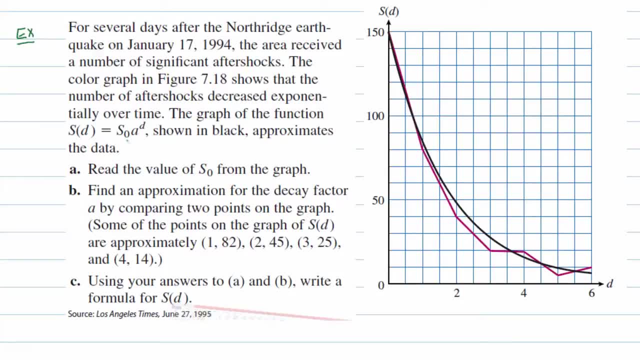 You can always change the letters in a problem if you want. They use S of D is equal to S, naught A to the D, And then they say it approximates the data. I probably would change that, mainly because I just dislike their lettering. 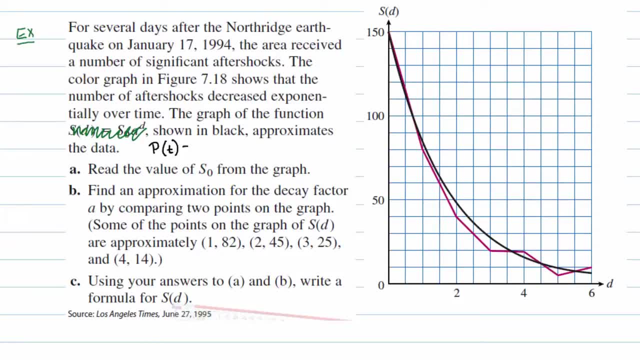 And I will go back to my P of T is equal to P And I will go back to my P. of T is equal to P, naught B to the T. Just because, well, I can do it, I'm allowed to. 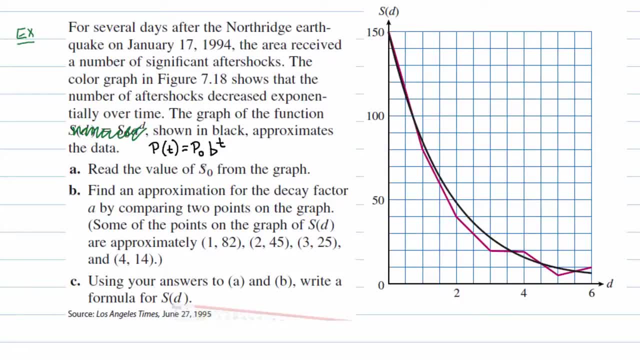 So are you? So? read the value of P naught from the graph. Remember, P naught is the initial value, So it looks to me that initially that's 150.. What that means is initially, on that very same day, there was 150 aftershocks. 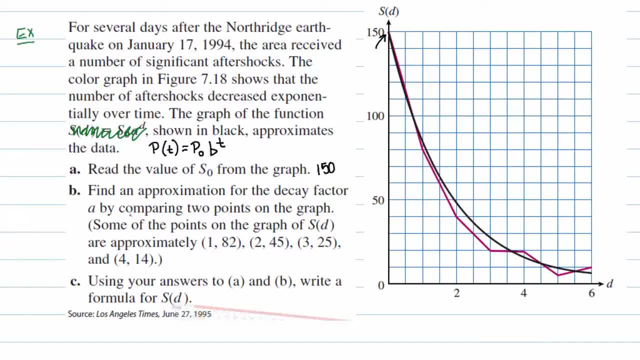 Find an approximation for the decay factor, which is going to be this B value, by comparing two points on the graph. Now you can select any two points that you want on the black curve, because that's the curve that we're going to use. 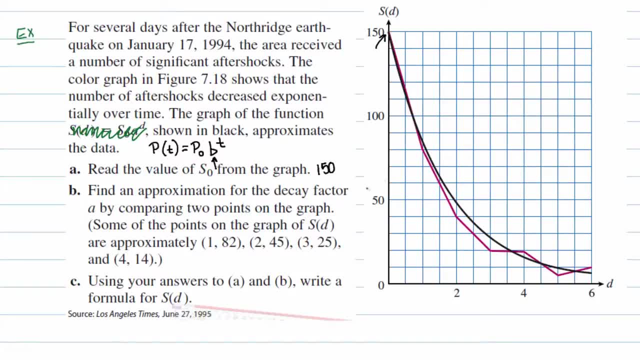 Although in reality you use if you're going to do some real data analysis, you don't. when he comes along and gives you this black curve, You actually have to select points on this red curve. So they're telling you. some points on the graph are approximately one comma. 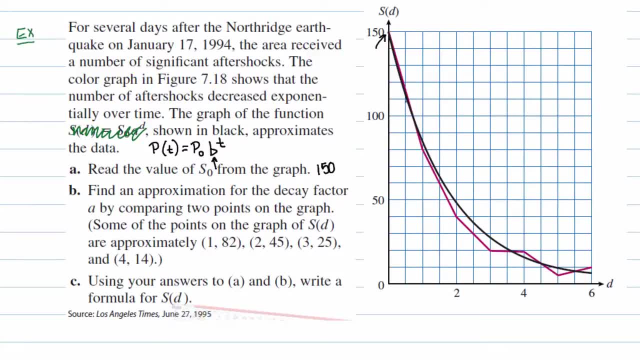 82,. so they're saying like: oh I see, because this is one right here, one comma 82.. So they're saying that this point right here is about one comma 82, and two comma 45.. 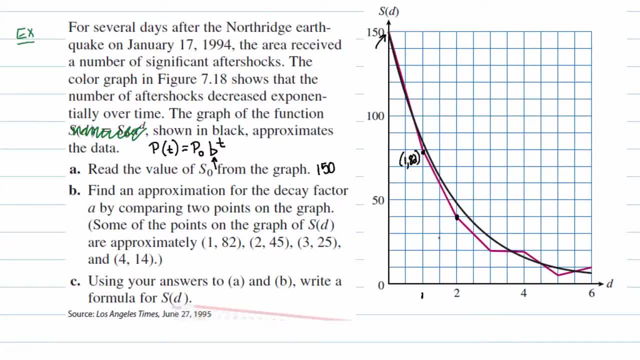 So they're saying that this is probably about 45. And in reality I think they're using the black curve, So they're kind of going in between these and they're saying that that is two comma 45. But, like I said, in reality 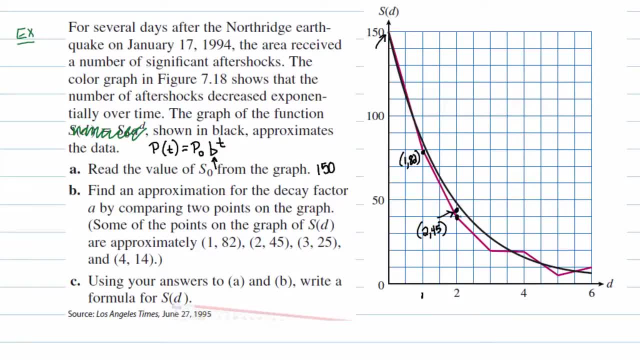 you would probably use the red curve Or maybe what they're doing here. maybe you should draw this curve along here and say, well, that looks like a pretty good fit. Let me just estimate in between what some points might be that would fit this data somewhat nicely. 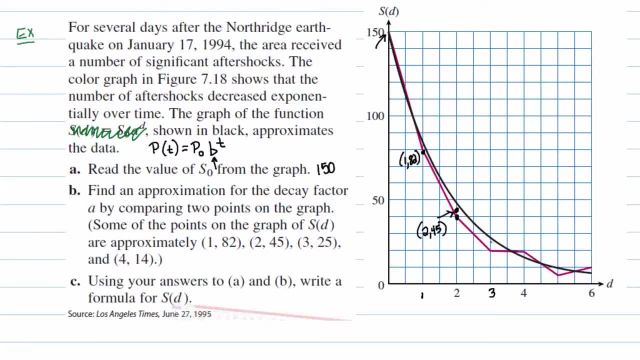 And they give you three comma 25, which is right about here, actually. And finally they give us four comma 14.. Well, that's 10.. It's actually a little bit higher than 14, but let's just say it's four comma 14.. 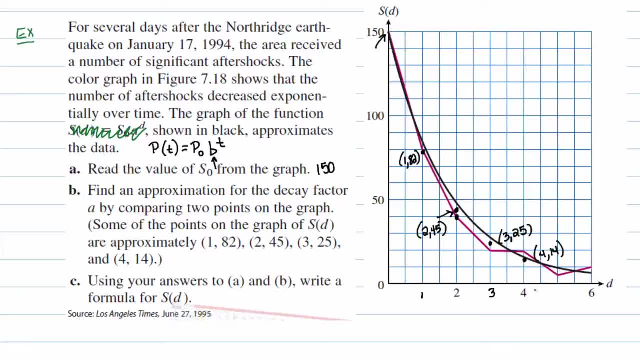 Okay, so they give me those four points. Now I could use any of those two points to determine the decay factor, Or I could use a calculator to actually get a better approximation to the decay factor. But I'll show you both here. 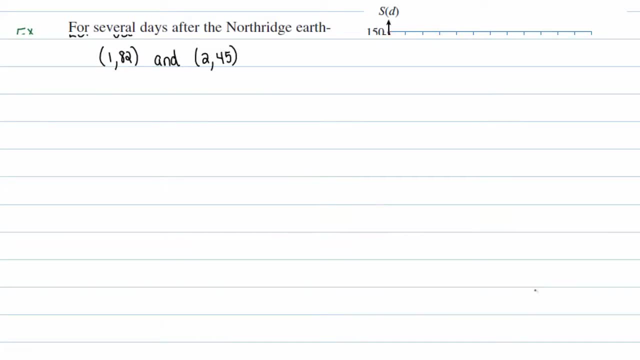 Let's use the points one comma 82, and two comma 45.. Now, there's a lot of fancy ways you can go about doing this, but the fact is that if your points are right next to each other, if you can set them up in a table like 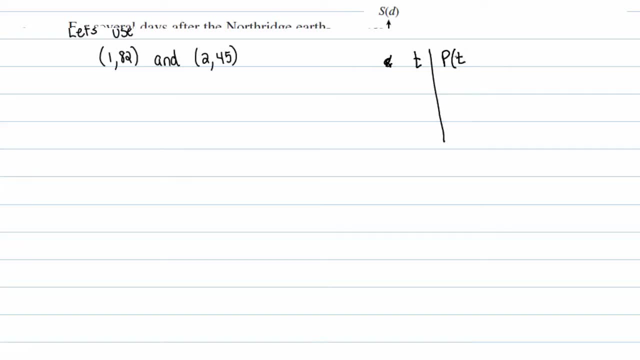 well, we're using Ts and Ps, so if you can set them up in a table and it goes one, two for your input values and 82, 45 for your output values, you can find out what the decay factor is just by noting. 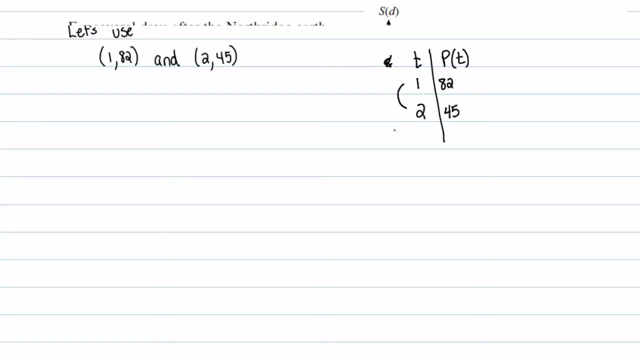 well, every time I step by one in the inputs, my output should be multiplied by some number. I don't know. I don't know what that number is, and I want to find out what that number is In fact. we're going to call that number B. 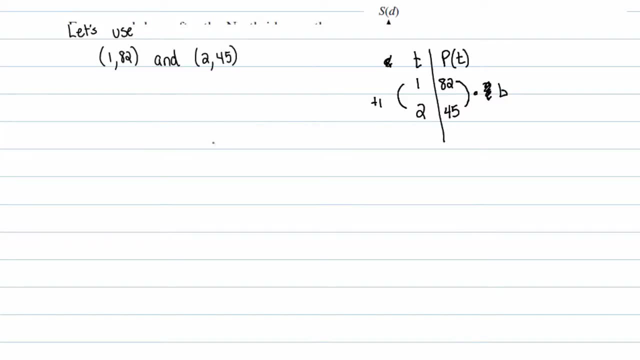 So it gets multiplied by some base. So let's see: 82 times what number is equal to 45?? Well, let's find out. Let's divide both sides by 82.. 45 over 82.. Let's see if that reduces. 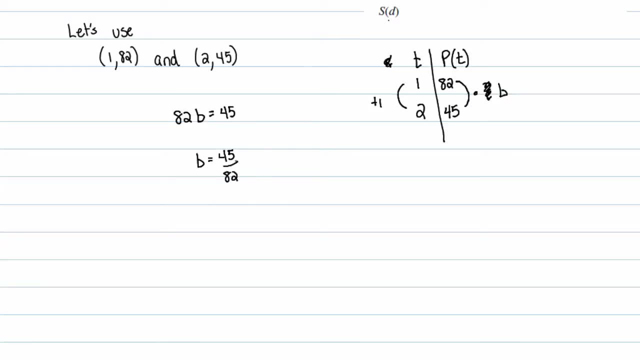 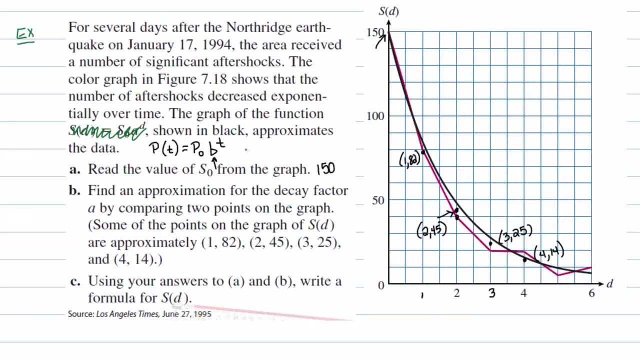 which it doesn't. I don't see anything in common here. So this tells me that the base is 45- 82nds. so let me go ahead and go back to the previous page. I see the decay factor is 45- 82nds. 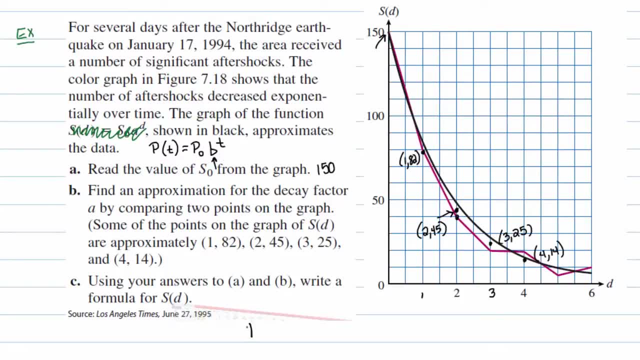 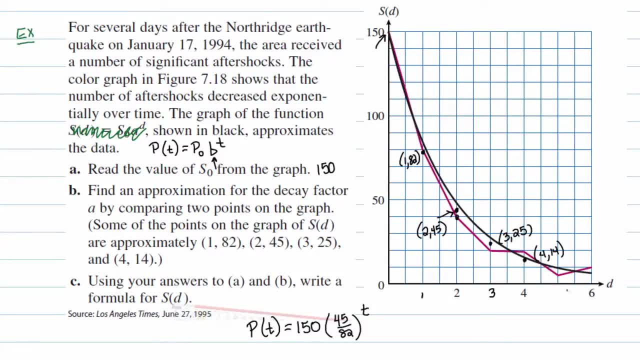 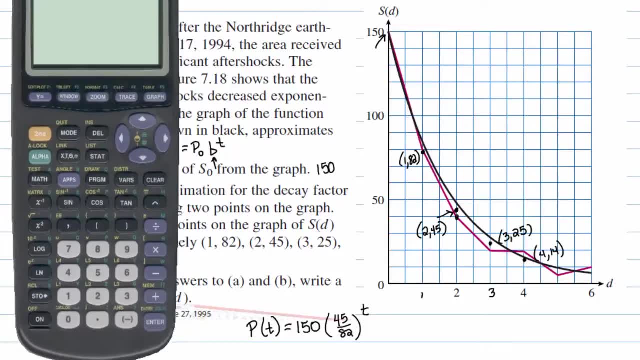 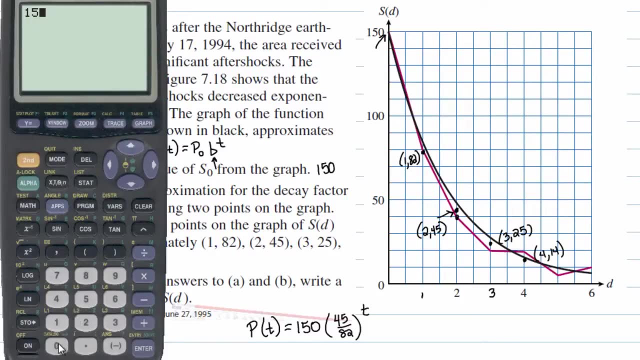 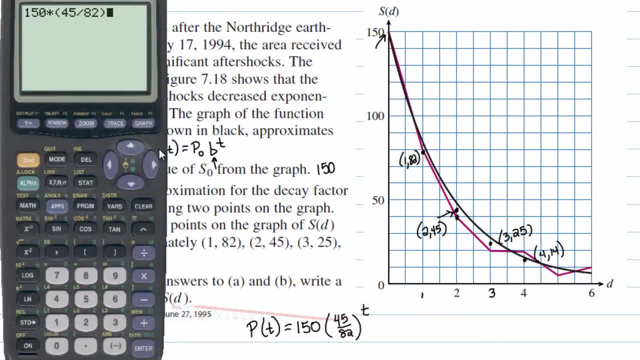 What time am I going to look for? Let's evaluate this at 3.. So I'm going to plug in day 3. And I'm hoping this will return something near to 25.. It won't return exactly 25, because in fact, 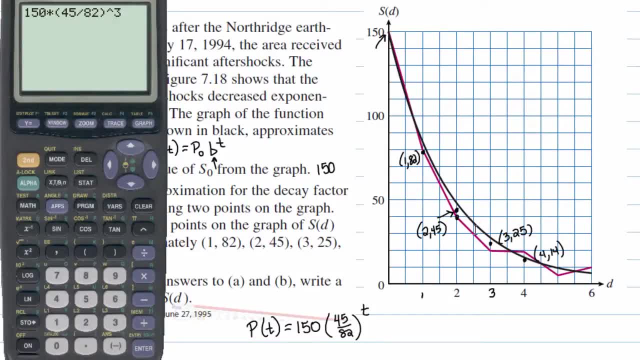 is. we're kind of just ballparking it here, but we're hoping that it will return near to 25 and it does, it returns very close to 25. so let me try that with day four and i'm really hoping that that returns something near to 14 kind of does. it's a little bit off, but hey, that's okay when we're. 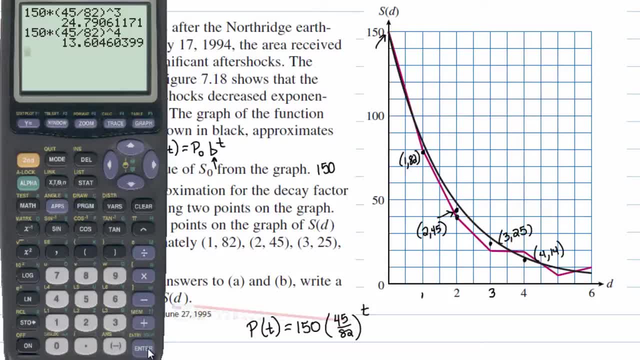 talking number of aftershocks and somebody says: you know you're rounding, that is 25 and 14 really. so that's a pretty good approximation, not too bad at all. now the other thing i want to do here. so i want to show you how you can really get some cool results using your graphing calculator. 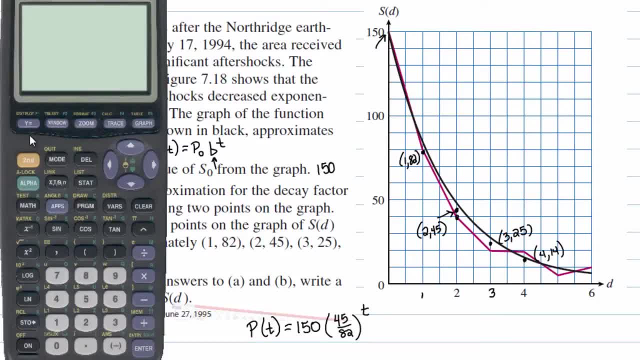 so i clear my screen. now get ready to learn. put your learning hats on. i'm going to first hit y equals and see i. i'm just going to clear out any of the functions i have in there already and let's type in the function that i've been given 150 or the function that i calculated. 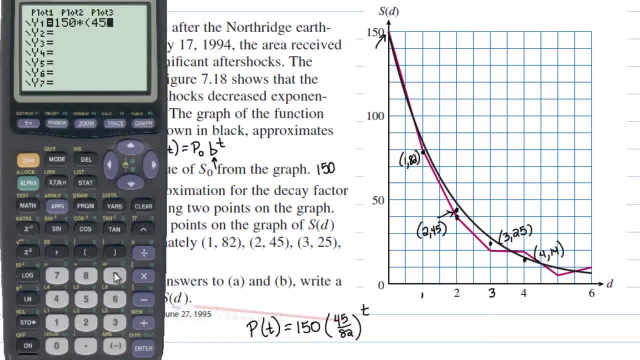 times the parenthesis, 45 over 82, and raise that to the x power- Okay, and I know it's supposed to be t power, but whatever, If you hit graph you're not going to see anything because, guess what, It's off your screen. 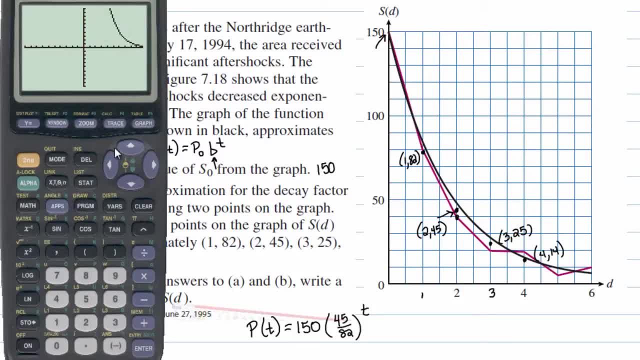 But that's well, okay, it's not totally off my screen. Actually, you see it right there, But that's not what I'm really concerned with. Well, I suppose I could be concerned with it. Let's adjust our window and say I'm not really concerned about anything. 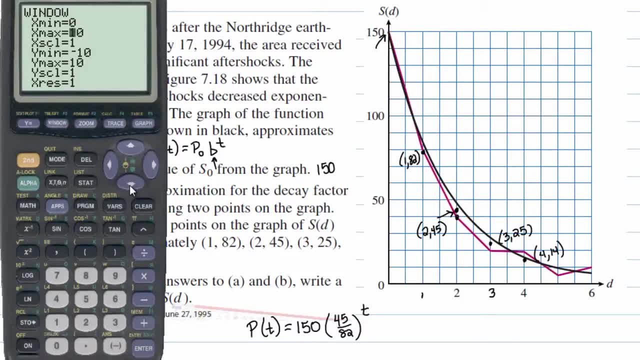 before the zeroth day And I'm going to try to match it up to their graph. I want to go up to the sixth day And let's see their graph starts at y equals 0 and has a y maximum of 150.. 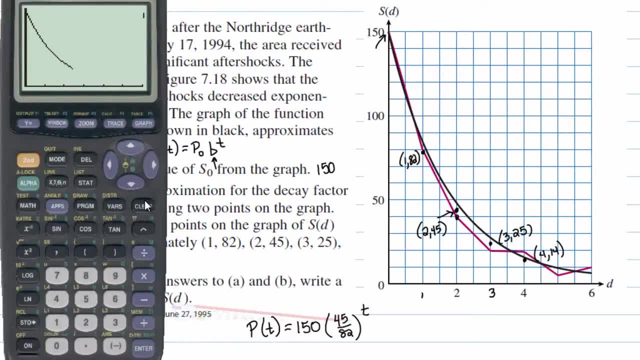 So let's see if my graph kind of looks like theirs. That's not too bad right Now. I've shown you some of these tricks before, but there's a lot of tricks you're about to learn, so get prepared. One thing: if you hit track, 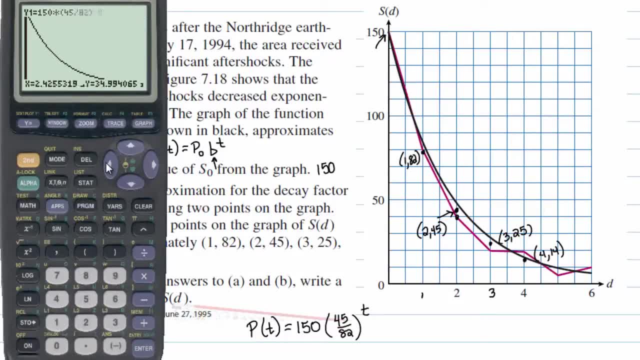 you can kind of go along this curve to the left and right and find out what x values give you what y values, And once you have hit that trace button, so once you have this x- y business down here, you can type in a number like 1, and hit enter. 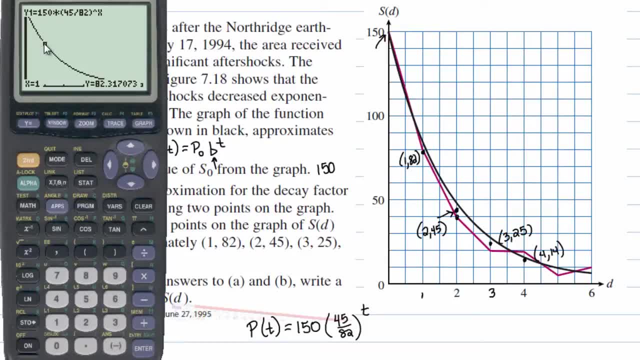 And it'll tell you: oh, when x is 1, the output's 82.31- blah, blah, blah, which is close to my 82. And when I type in 2, the output is 45.17,, which is close to my 45.. 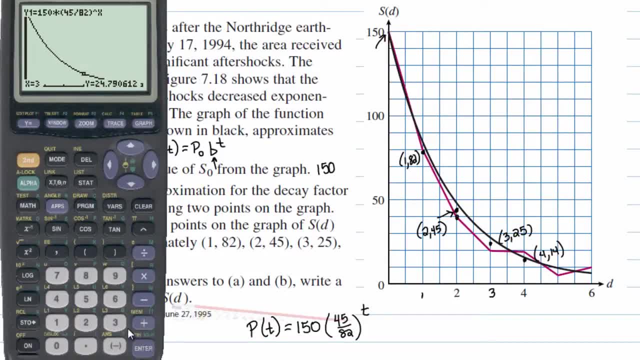 And when I type in 2, the output is 45.17,, which is close to my 45. And when the output is 3,, again we know that's 24.79.. When the output is 4, the output, or when the input's 4, the output is near to 14.. 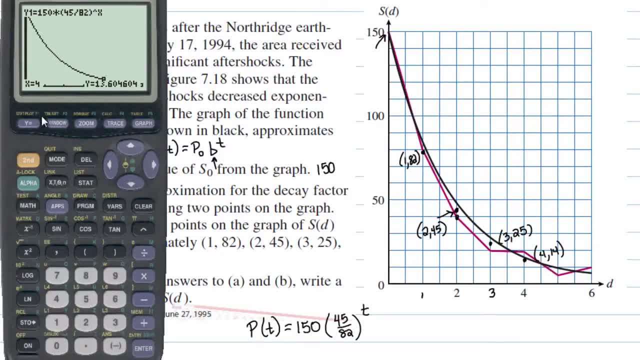 So this is a really cool way that you can get all these values. You could also look at them in a table. So if I hit second notice, I hit the second key and table menu is right above the graph button, so hit graph. 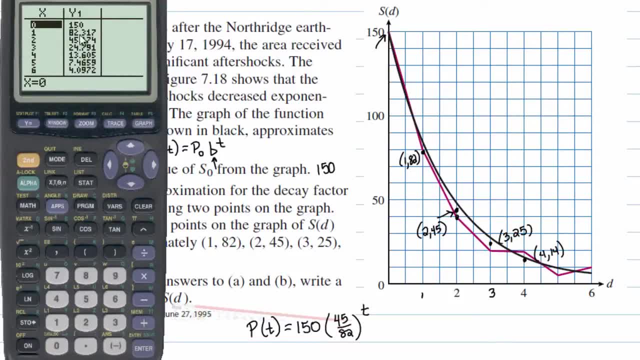 You get a bunch of x values and a bunch of y values. Now yours might be different, so let me set yours up. for you To set the table, you have to go to the table set feature, so hit second window to access the table set. 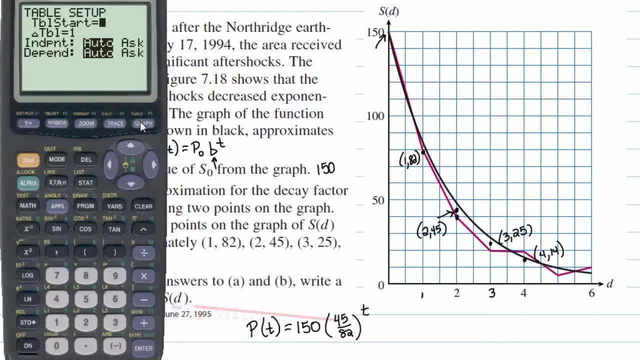 And this just asks you: hey, where do you want the table to start? Zero's a perfect place. What do you want to increment by Delta? capital? delta there means increment or change in the table value, So I don't mind it changing by values of 1.. 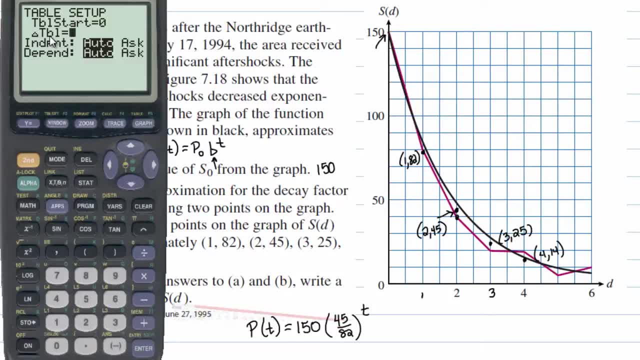 You know going t, t equals 1, t equals 2, t equals 3.. But what's important to me actually is this business down here. I want it to ask me, I don't want it to automatically create a list. 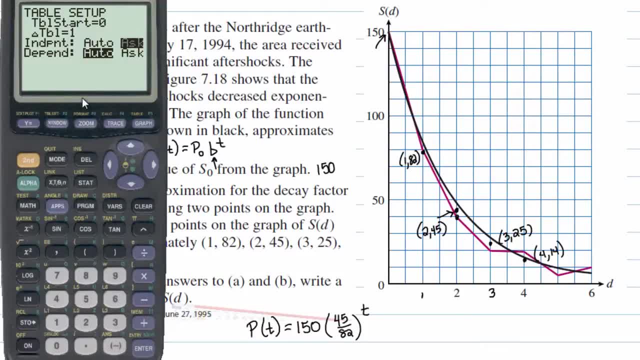 I want it to ask me what I want to plug into my function And I'll let it automatically figure out what the answer is. So now that I've done this, I'll hit second table again. Notice my table's empty, but I'll plug in zero. 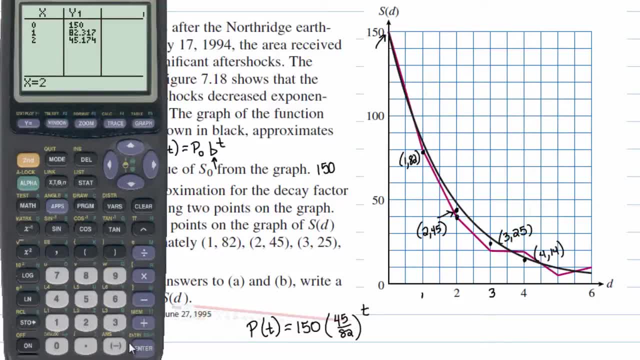 And then one, And then two, And then three. See, notice, this is giving me the same values, but it's just really clean, Very nice. So you see, like, for example, after six days there were only four aftershocks. 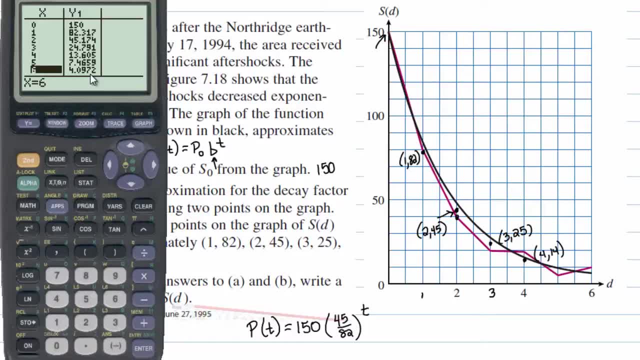 Always keep in mind the application you're dealing with, because that interpretation for the applications is super important. Now, if you thought that was a lot, it wasn't, Because all I really told you how to do is, well, graph a function. 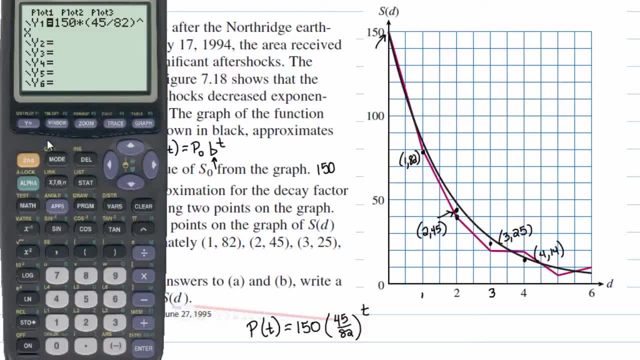 which I've told you how to do in the past, and how to look at a table and build a table of values, which I've told you how to do in the past, And I told you how to use the trace button and to go to an exact point on the graph. 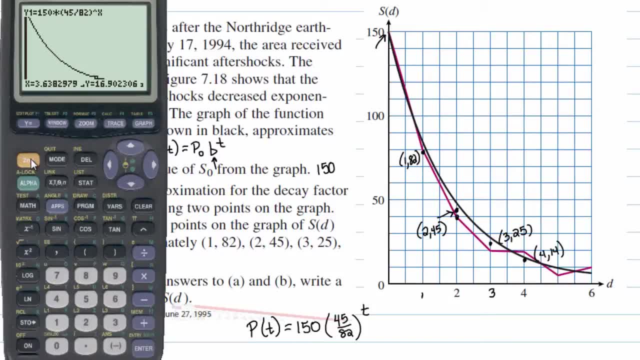 which I've told you how to do in the past. So there has to be something new. I'm going to teach you, And you're absolutely right. We are now going to make a group of statistics, Not like averages and means and medians and modes and stuff like that. 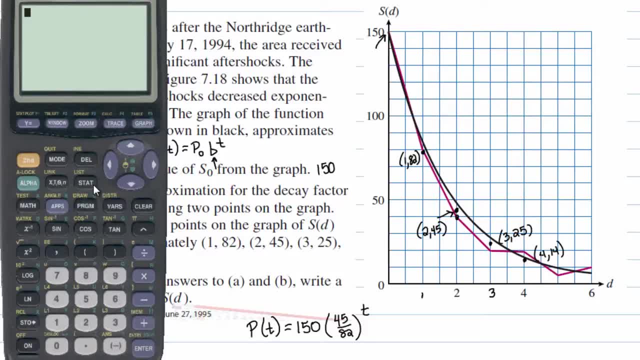 but a list of data. So you see this stat button here. If you're given a real situation where somebody says, hey, here's a bunch of data points, I need some type of function that fits this, Then this is the button, the go-to button. 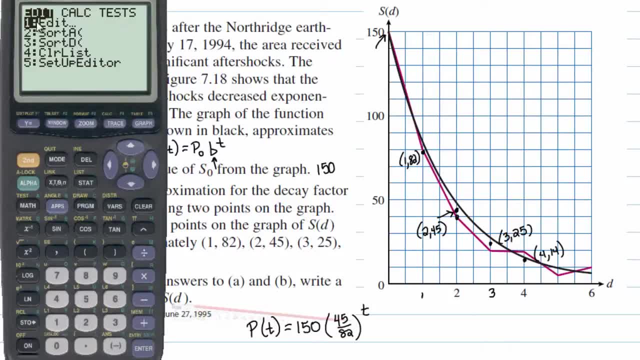 You're going to hit stat and notice all these submenus. You have an edit menu, a calculate menu and a tests menu, But the edit one is what we're going to work with initially. We're just going to edit. We're going to edit a list. 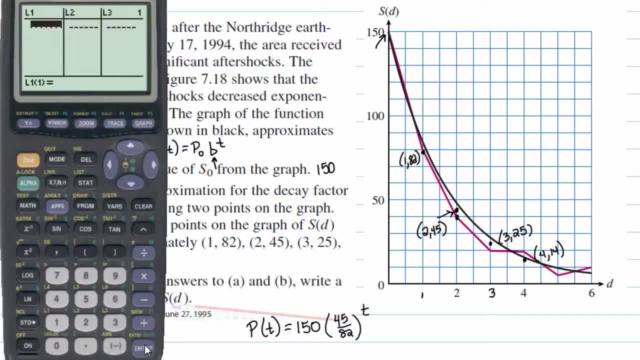 So just select that first option there. Here's my list menu. I have list one and list two. In list one, I'll call those my x values. In list two, I'll call those my y values. So my x values are zero actually. 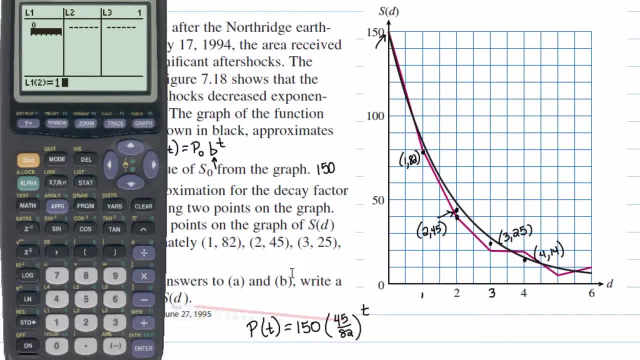 Sorry, I typed one, but I meant zero. Zero one, two, three and four. In my y values, or my outputs, I had 150.. By the way, that was my guesstimate that it was 150.. 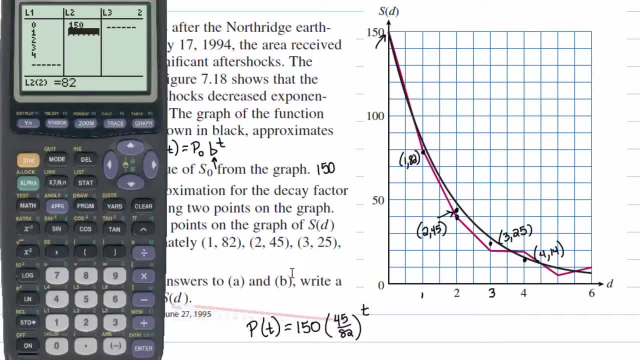 It looked like 150.. Eighty-two, forty-five, twenty-five and fourteen. Very important that those two lists be of the same length. Now, really, right now, there's nothing that I can really say. It's not going to do anything for me just to have this list in here. 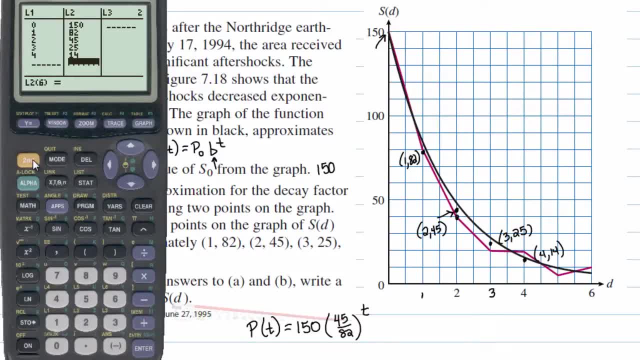 But let me quit out of this menu. So, second, quit, Back to the main screen, the home screen, And I'm going to go back to my y equals here. My function's right here. See this little top menu that says plot one, plot two, plot three. 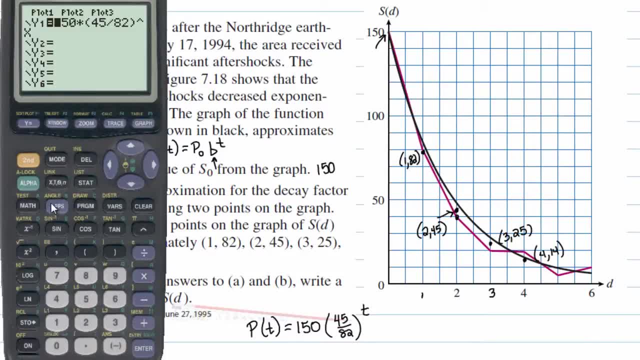 That's where you can turn on your plots, And I want to plot these points. So what I'm going to do- you can either go up here and just hit enter, or you can exercise a little more control and hit second. and hit y equals. 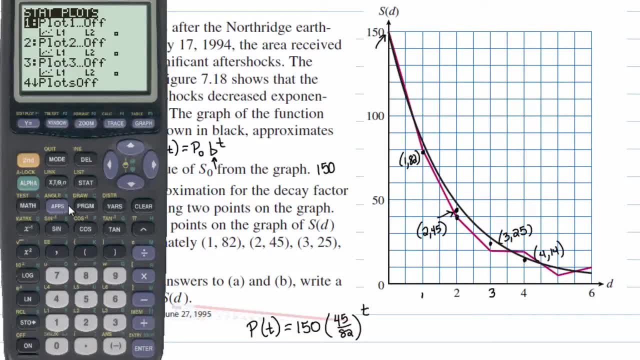 When you hit second and y equals, it accesses the stat plot menu, Because we're going to plot a bunch of points. let's use this Now. I'm going to just use this If you're only going to. it's like the function menu. this y equals thing. 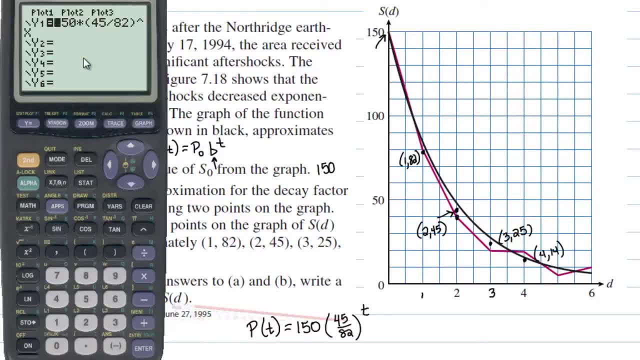 There's no point in starting writing an equation in y four if you haven't filled up y one, two and three yet. So same thing in this menu. There's no reason to use plots two, three or whatever if you haven't used plots one yet. 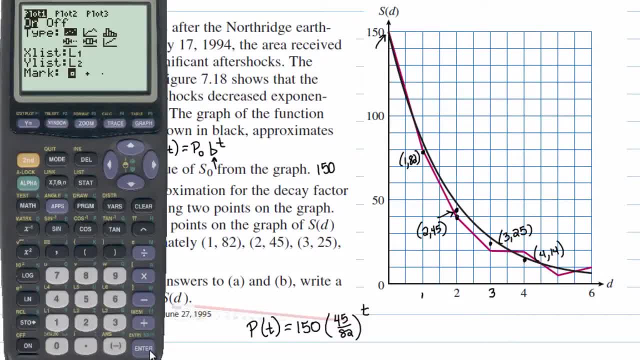 So let's use plots one here. Click enter, I'm going to turn it on. It's automatically set for a scatter plot, In other words, it's going to plot points And it should automatically want your x list to come from that list one. 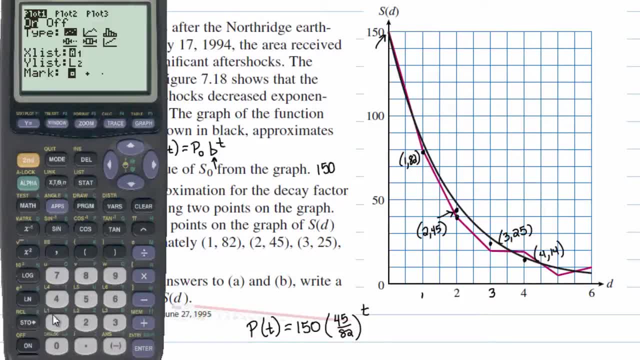 and your y list to come from that list. two: If it doesn't down here on your keyboard, you see the number one Right above it is an l one. You would hit second l one. Okay, Same thing for l two. 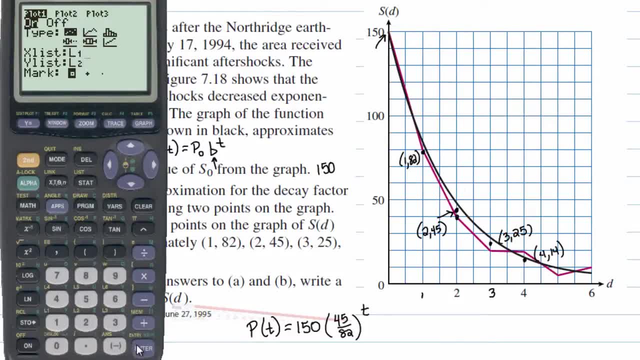 You do second l two, if you needed to, And then you can just go ahead and hit graph And look, it has my points on there. Look how nice that fits too. Very, very nice curve. If you have a bad, a hard time graphing or getting the right size window. 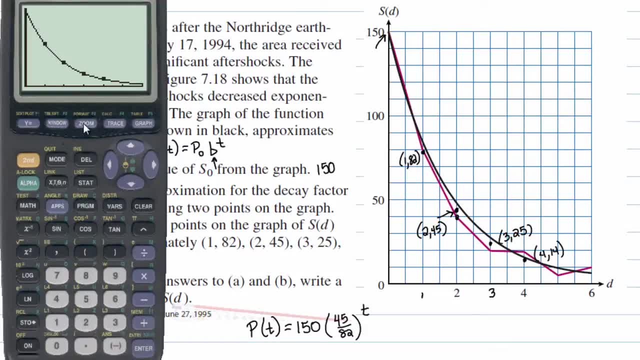 if you have data points already, you can actually hit zoom. And if you scroll down quite a bit, the ninth option is to zoom to your statistics. If you hit that it'll zoom to a window that exactly fits your data points. You can see in this window. now I've zoomed in a little bit. 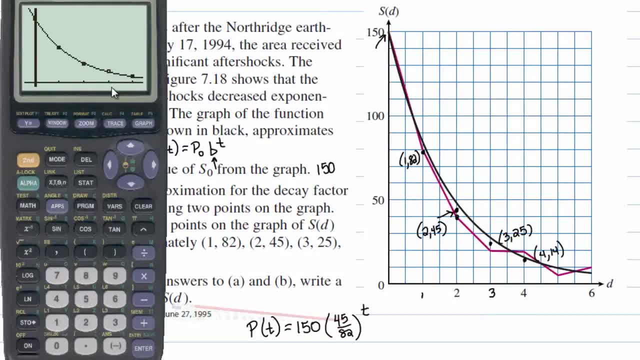 I notice that x equals three. it's not the perfect fit. So is this all you can do? And the answer is no. Let's recap really briefly what I've told you to do: Graph a function. You already know how to do that. 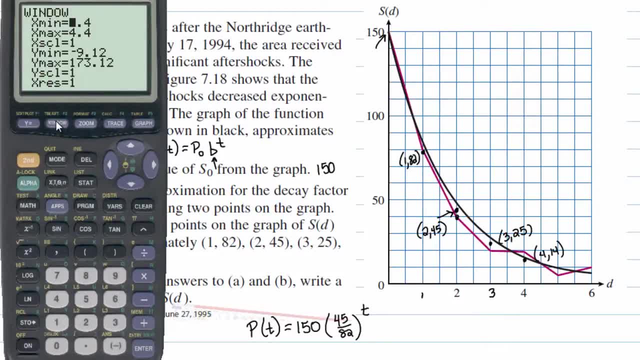 Just type something in hit graph and there it is. I've told you how to adjust a window. but we know how to adjust a window. I've told you how to zoom on things. I've told you how to trace along your graph. 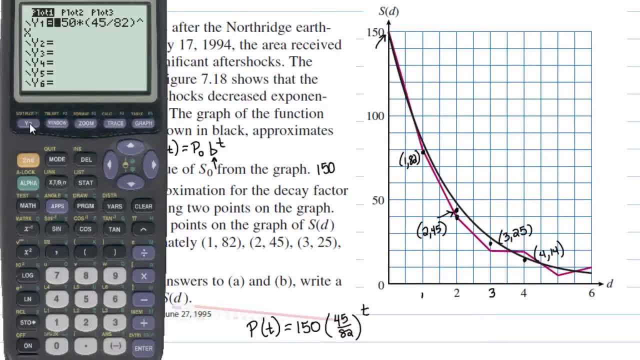 Okay, But now, oh, and I also told you how to enter in a list of data through the stat button, Hit stat edit, and then you can enter in your list of data And then to plot that data, you would just go to stat plot. 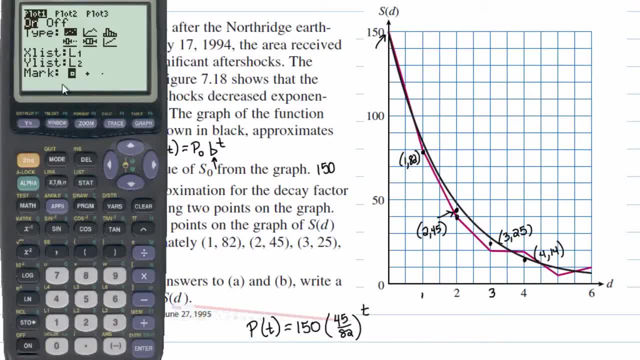 So second stat plot here, and you could turn those on. So this is all I've told you to do. It still seems like quite a bit. Now, if you are not faint of heart, let's try one last thing, And this last thing is probably the coolest. 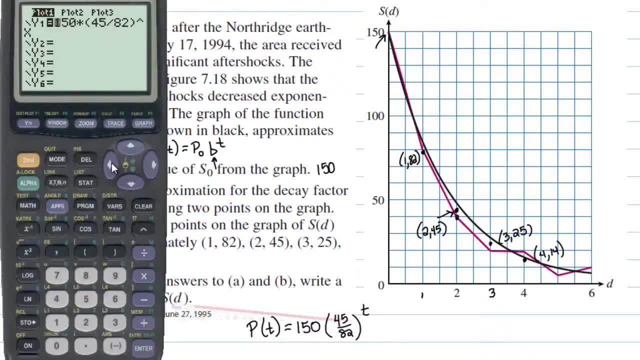 Anyway, what I'm going to do is I'm going to go ahead and delete our function here, So it's no longer there. If I hit graph, you'll see All I have are points, And what I'm going to do is second, quit and go to the stat menu again. 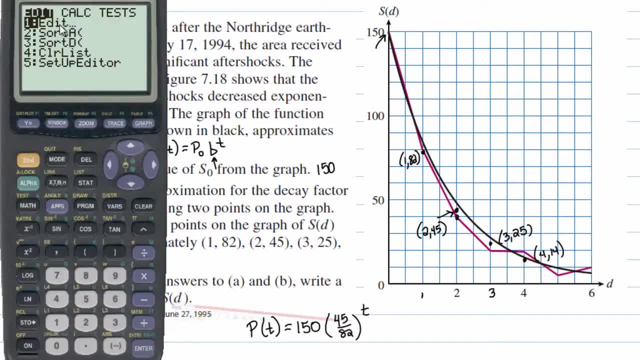 Remember I've already had, I already have a list one and list two with my X and Y values. Now I'm going to calculate. hop over here. I'm going to calculate a regression curve, And this will be what a calculator does is it gets you the best possible curve that will fit to this data. 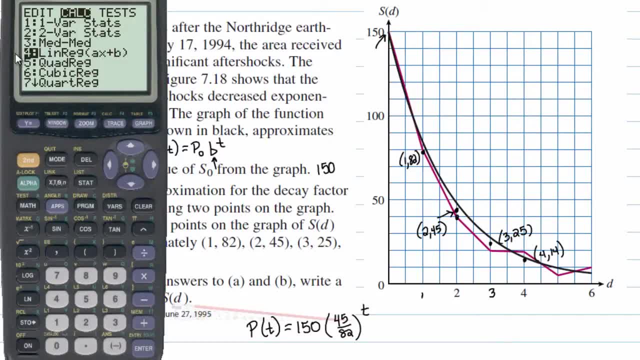 And you get to actually select what type of curve it is, So you could select A line. Try to fit a line to all four of these points, which is not going to happen. You try to quadratic function or a cubic function or quartic function. 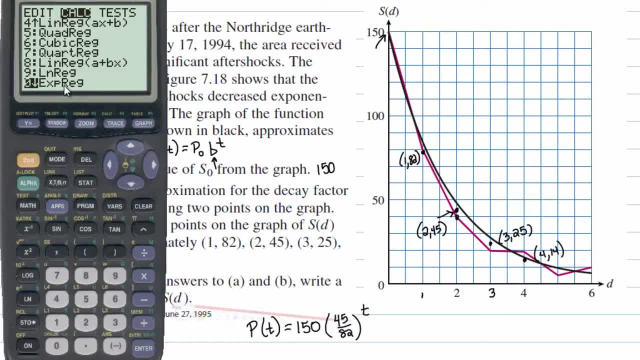 But I'm actually going to do an exponential function because we're in, we're talking about exponential function, So I'm going to go ahead and select that. So again, it's under your stat menu. You select calculate, because you want to calculate a regression curve and select. 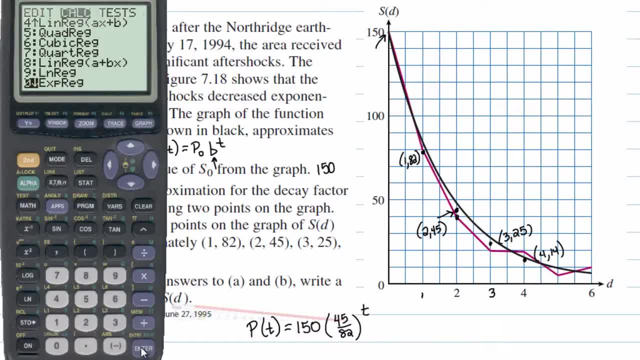 Exponential regression or X reg. hit enter and it doesn't look like anything happens. The reason why is it's expecting you to tell it where your X values are stored and where your Y values are stored. As long as you stored them in list one and two, it automatically assumes that's where you want. 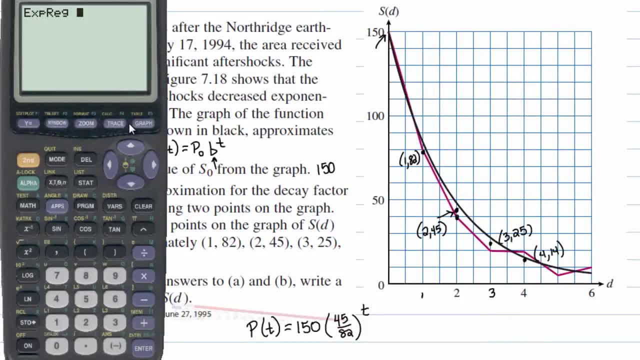 So if you hit enter again, it'll give you the perfect regression equation. If you don't, if you didn't store in list one and two, if you stored in list three and five or something like that, then you could label them here. 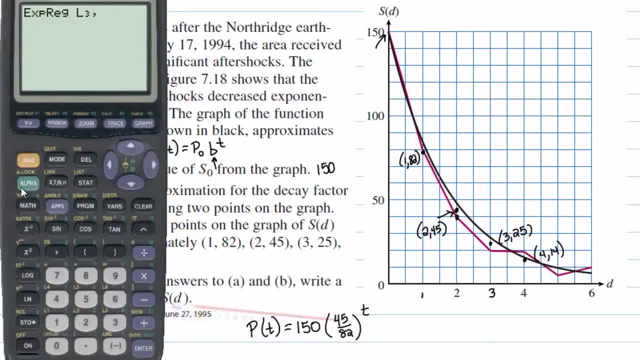 You could say second list three comma, second list five, But in my case I did list one and two, So let me go ahead and delete these out of here and just hit enter because, like I said, if there's nothing entered, it'll automatically assume list one and two. 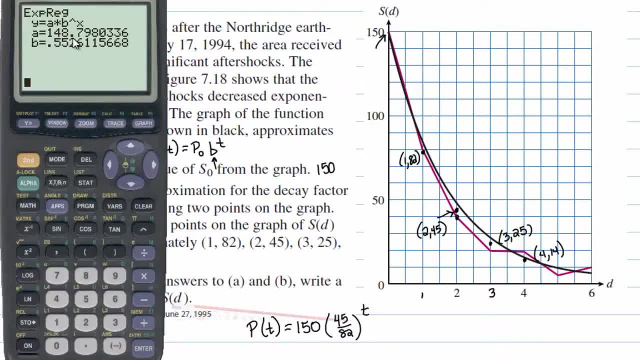 So here's where our it says the perfect function is 148.8 for the co-occurrence. So here's where our it says the perfect function is 148.8 for the co-occurrence. So here's where our it says the perfect function is. 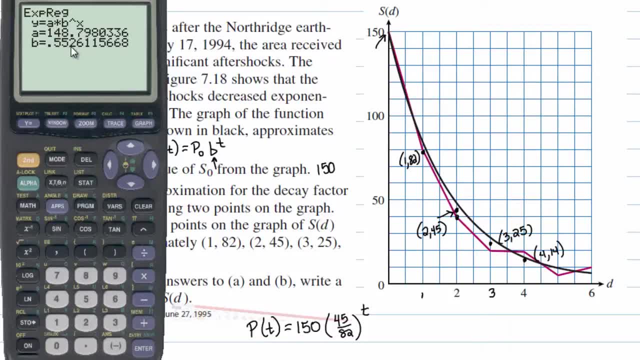 148.8 for the co-occurrence- It's a coefficient or the initial value- and 0.5526 for our base. I wonder how close that is to this. I can't remember what this was. So the base that we had calculated was 0.54878.. 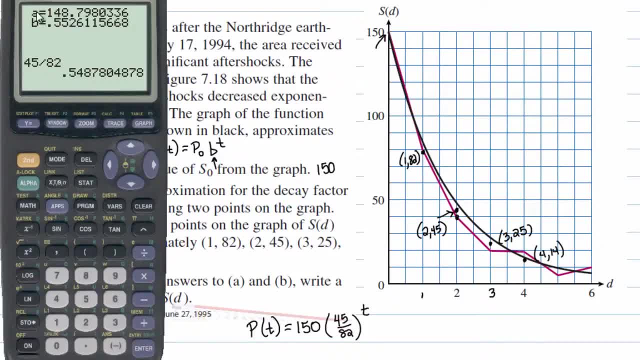 That's very close, But let's go ahead and use the function, the exponential regression function. Remember the P naught for that. the calculator got was 148.8 and the base is 0.5526. now do you want to type in all those things? 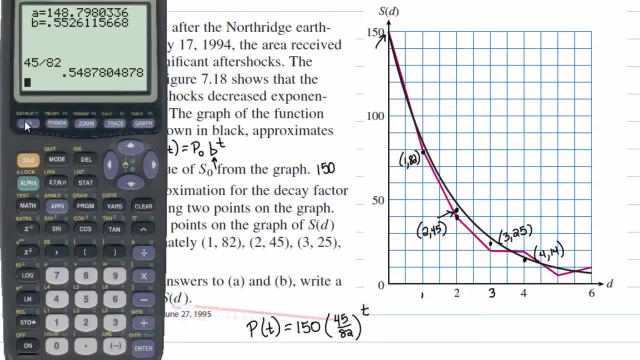 probably not. you could, if you want to. you totally could. you go to y equals and you could type those points in or those values in. but i will show you a better method. first thing you do is- and it doesn't matter if you clear your screen or not, i just like to clear. 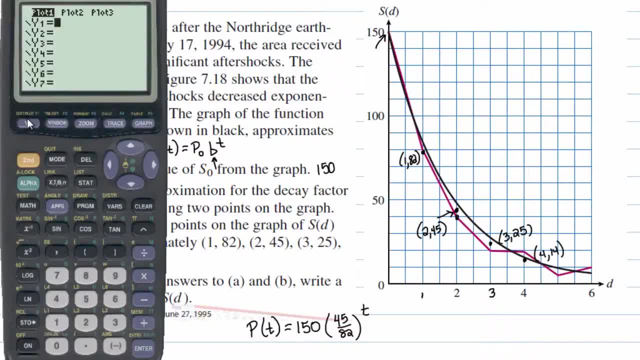 my screen. first thing you can do is you want to, up here, hit y equals. so you're in the function menu, the graphing function menu, and you're going to insert a variable here. so i'm going to go to the vars button. it's the only time you're likely to use this, so just watch. it's pretty neat, you. 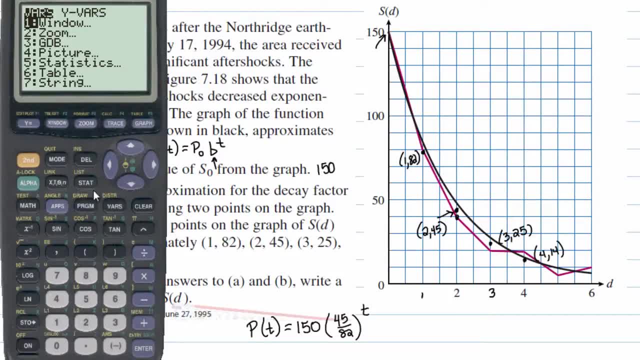 know the vars and there's a lot of weird things going on here, but i just did something with the statistics. i know i did something with the stat menu, so let me go to that. that thing, that might be a good thing. so, vars and you, stats and man, there's just too many choices. i'm overwhelmed. oh, but wait a second. i just made an. 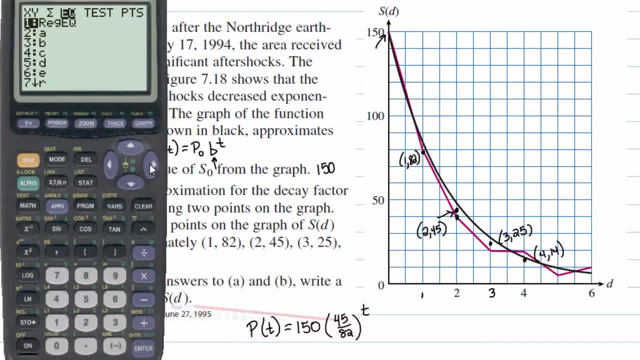 equation. there's an eq right there. maybe i should go over there. oh, look at that reg eq. if i hit enter, it will automatically insert the right regression equation that i just calculated. so again, the key strokes are: let me clear this uh line out so you can see it again, although you could rewind, so i 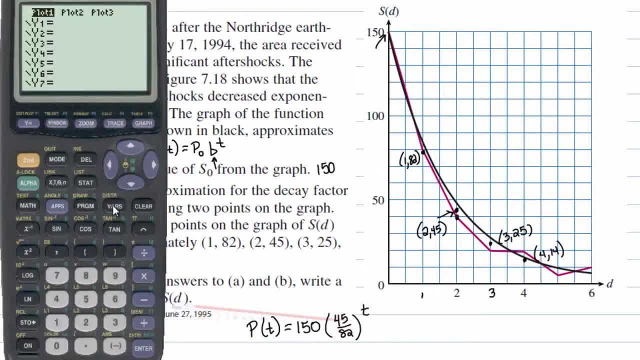 don't know why i'm saying that. uh, you get to this y equals menu. hit vars to the variable. we're working with some set of statistics, so select that and you want to insert an equation, specifically the regression equation. now, if you hit graph, this curve is the perfect curve to this data. 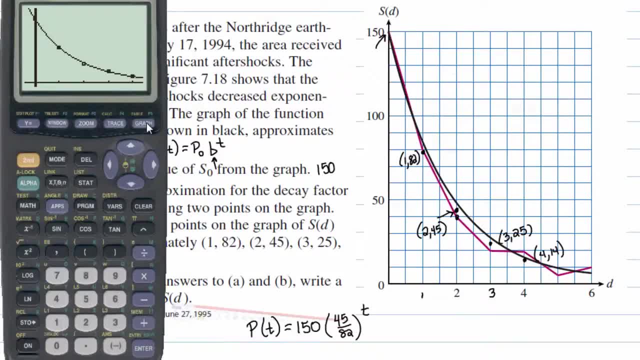 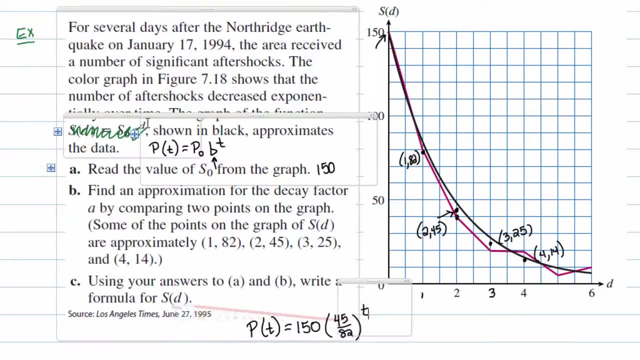 and then you can make predictions and use this function for other things: predict how many quakes 10 days from now. that type of thing Pretty neat, And that'll about do it for solving exponential equations without logs.